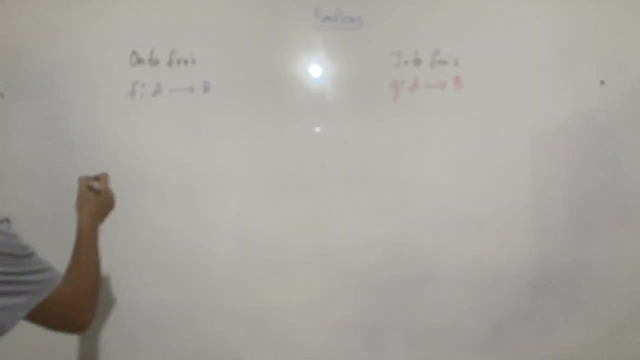 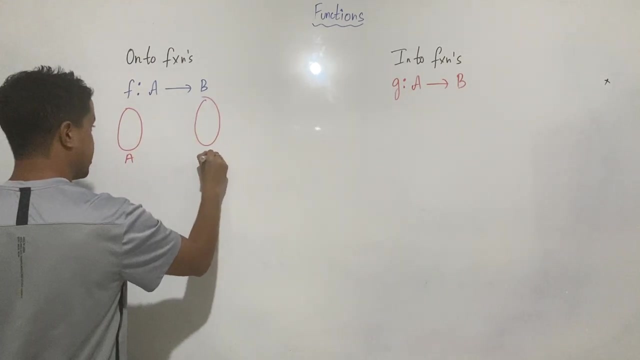 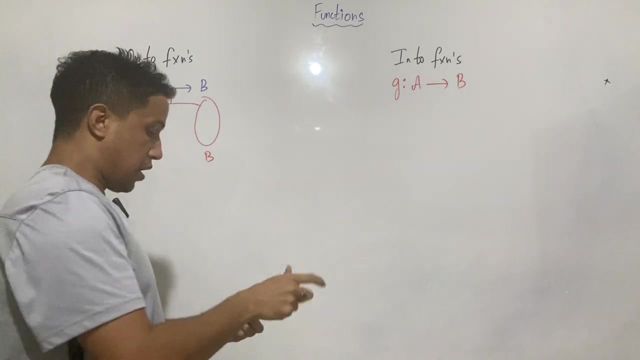 from set a to set b. okay, So here this is my set a, this is my set b, and here the function f is defined from a to b. okay, Now, here in a I have, let us say I have here. 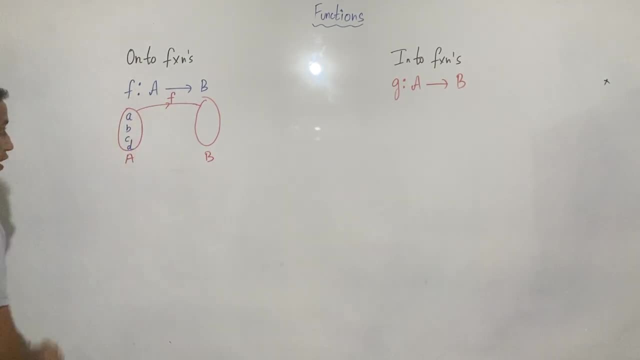 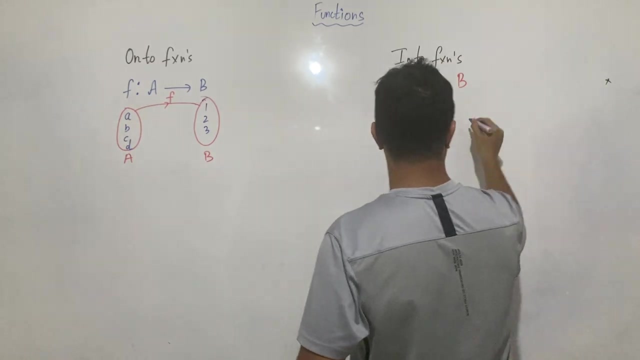 four elements: a, b, c and d. okay, And in set b I have three elements: one, two, three. okay, So same I will do here. here: this is set a, this is my set b and here: 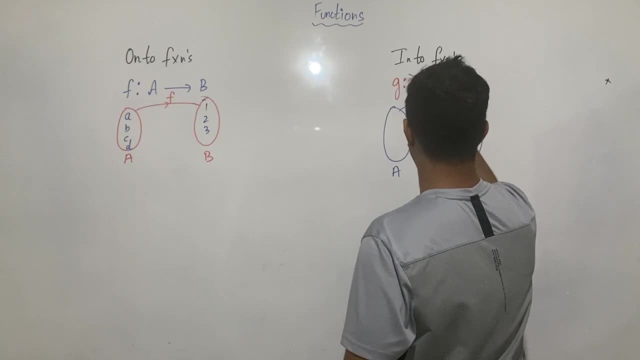 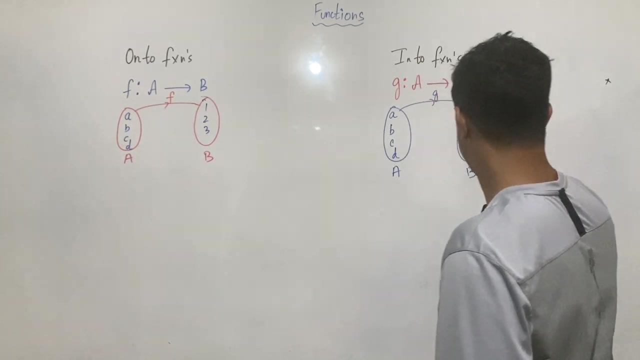 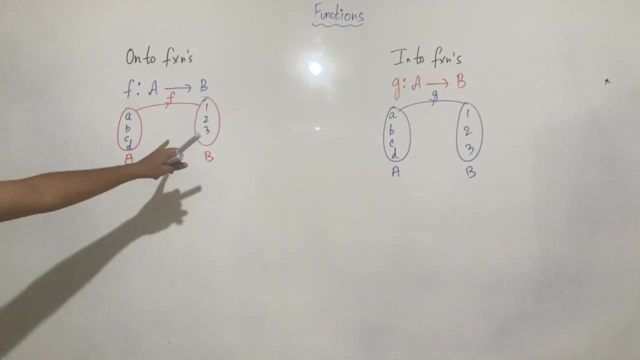 the function g is defined from a to b. right Here I have four elements: a, b, c, d and here three: one, two, three. okay, Now see here. now you have to observe a few things. 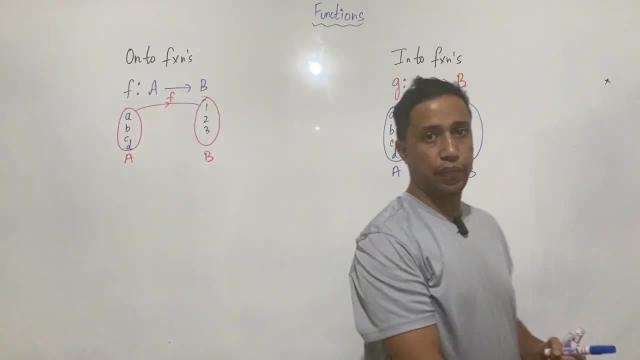 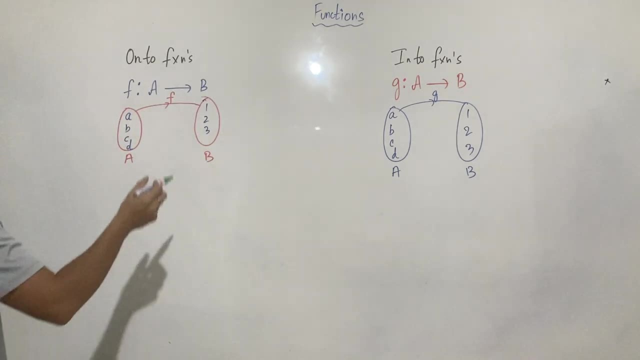 okay, Now I am going to map the elements on the left with elements on the right. okay, Let us say that a is mapped to one, okay, b is mapped to two, c is mapped to three and d is also mapped. 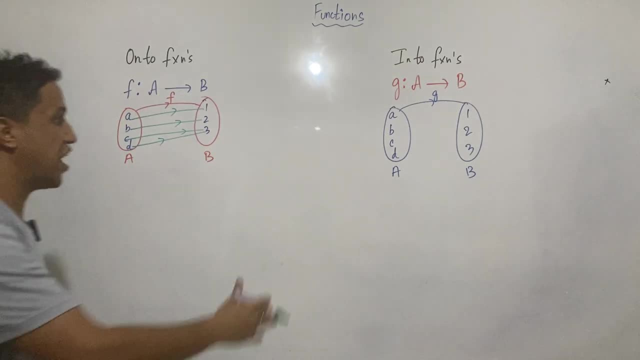 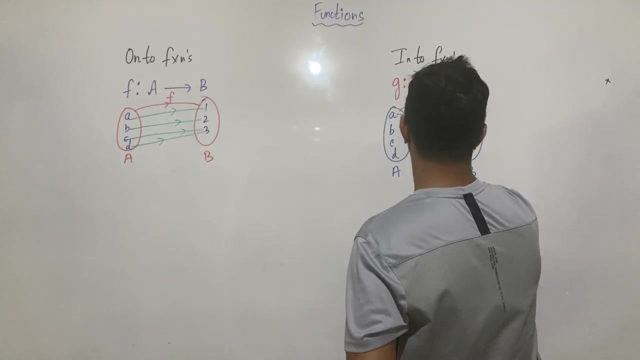 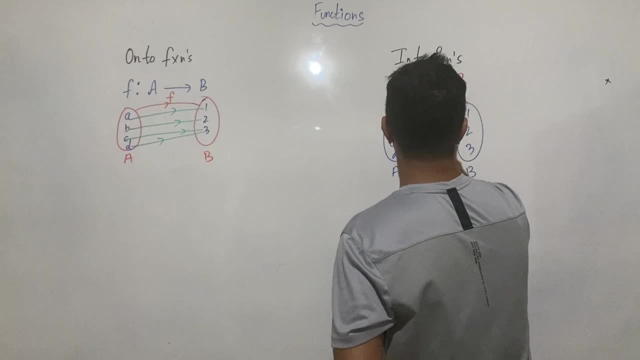 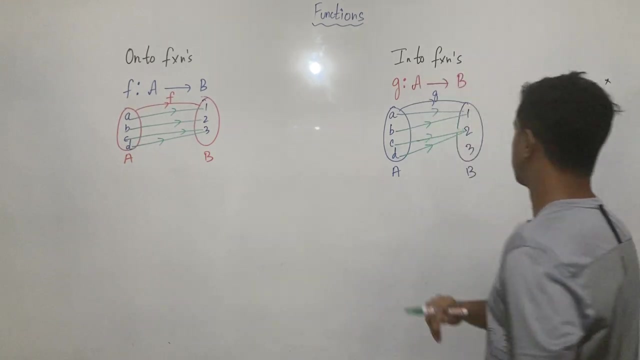 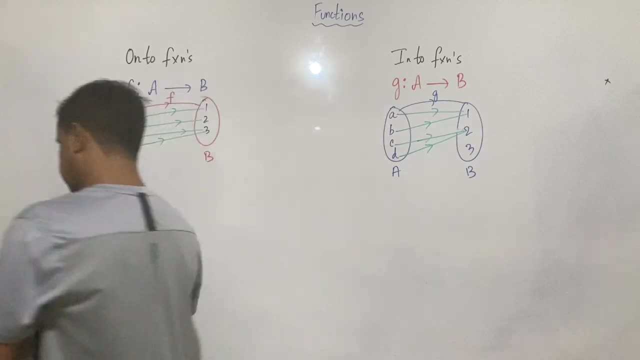 c is mapped to three and d is also mapped to three. Okay, Now come to both the cases. First come to ONTO function. When we say f means f is a function defined from A to B. it means that here my A is domain. 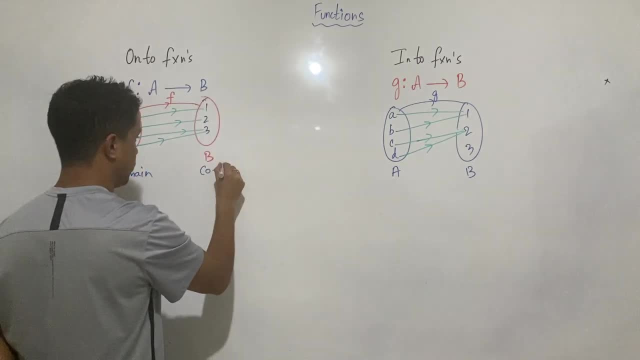 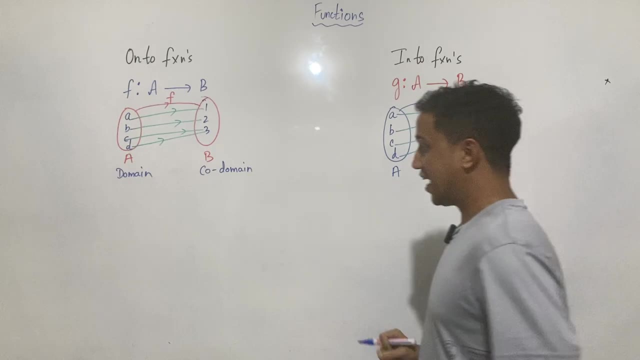 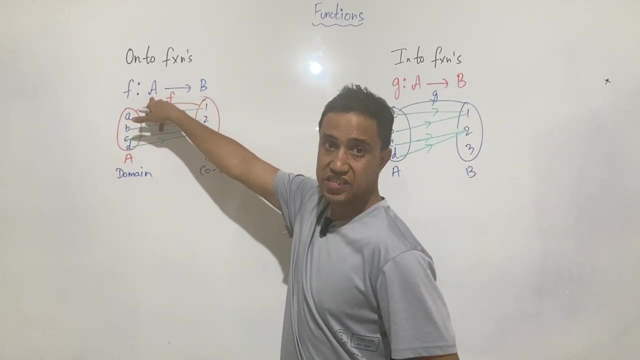 and B is domain, so it is a domain. That's the domain I create here. That's the domain I create here, Codomain. So whenever the examiner or anyone gives you the function, then you have to figure out the domain Domain. it's going to be this and: 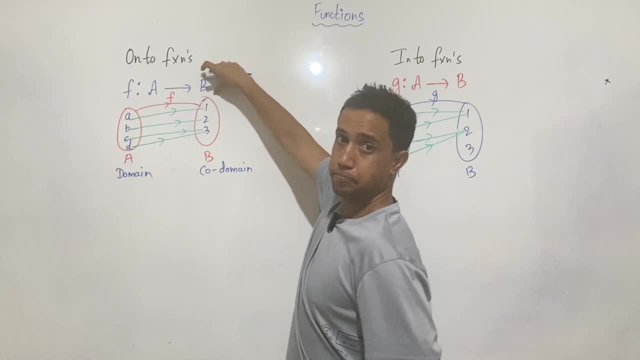 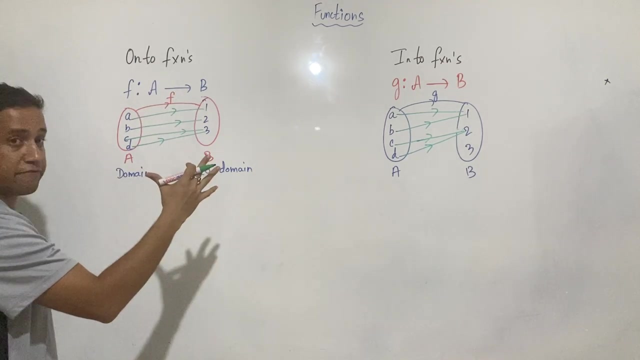 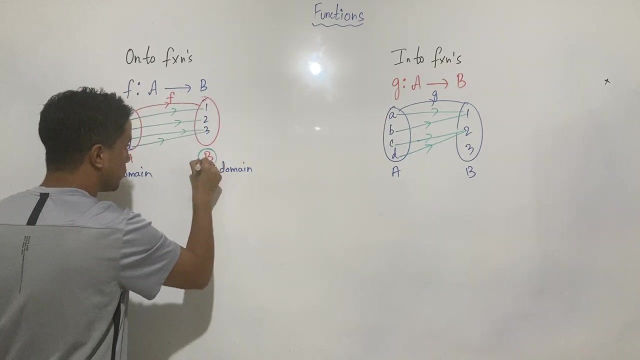 this is going to be your codomain, So please put this thing in your mind. Now, if you look at the mapping, and especially when you look at the elements of the codomain here, you can see that whenever we have to classify functions as onto and into, our main point of focus must be our codomain. 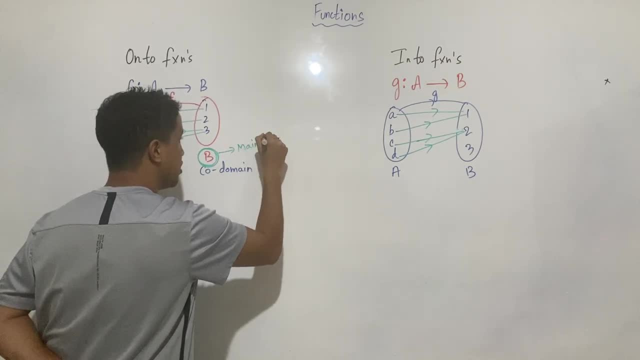 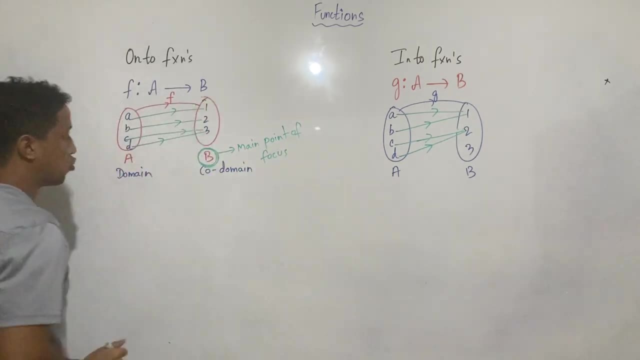 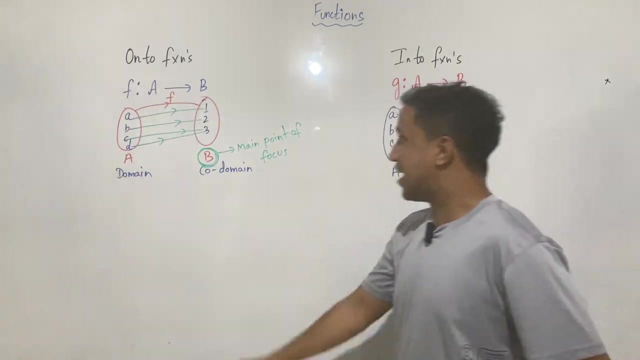 This is the main point of focus. Now you look at elements in the codomain. Now look at one. Does one have a pre-image? Yes? Does two have a pre-image? Yes? Does three have a pre-image? Yes? So when all the elements in codomain have pre-images in domain, 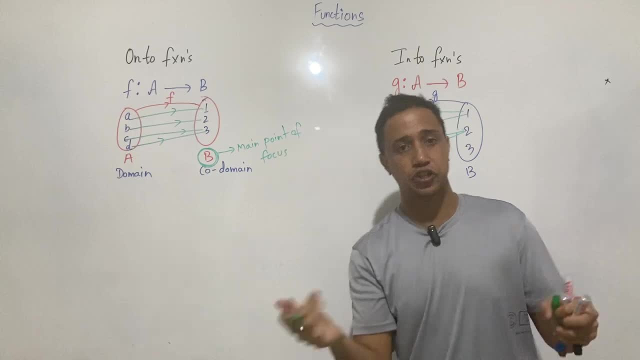 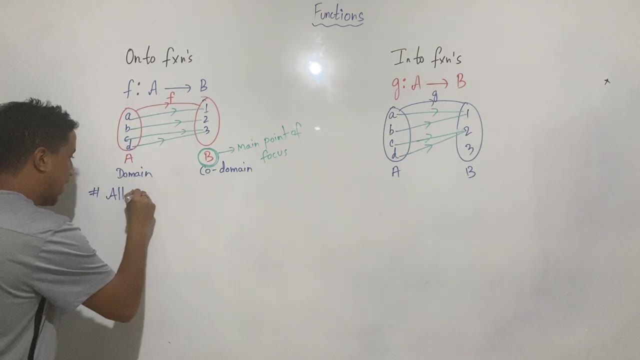 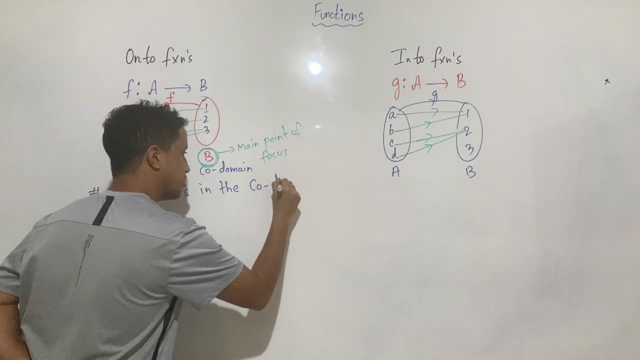 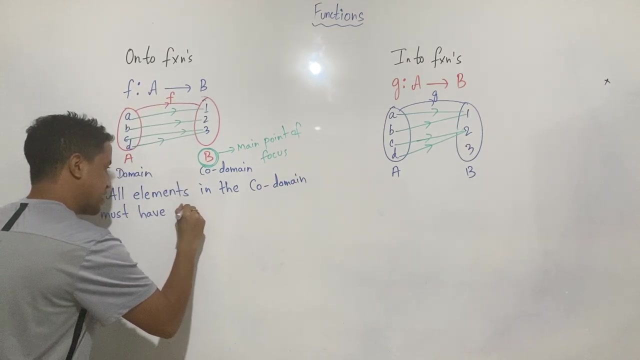 then that kind of function is known as a onto function. So here you can say that all elements, elements in the codomain, must have, must have, pre-images in domain. Okay, So if that happens, then your function is going to be known as onto function, onto function. so this is the main thing. okay, if the elements, if all the elements, 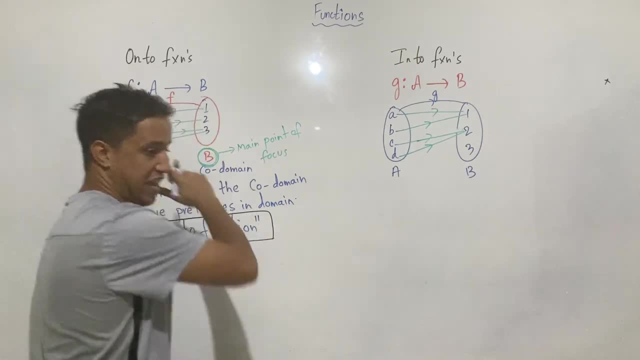 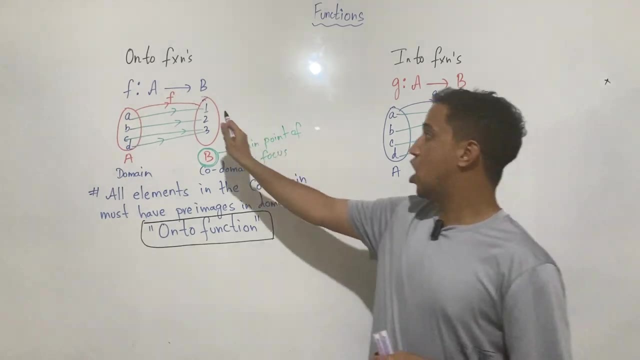 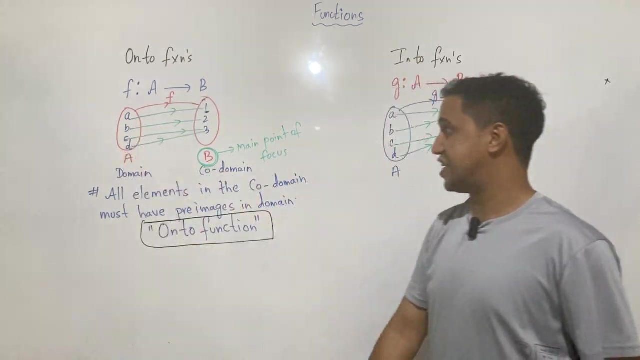 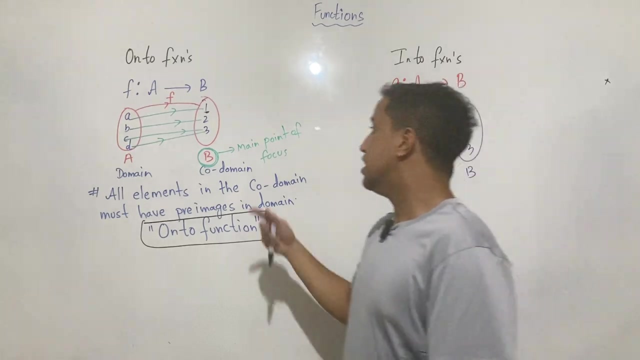 in your code domain, have image or have pre-images in domain, then it's going to be your onto function. one has pre-image a, two has pre-image b, three has two pre-images, c and d. so all the elements have pre-images, right? so this is onto function. now, if you look at the the code domain here now, see here: 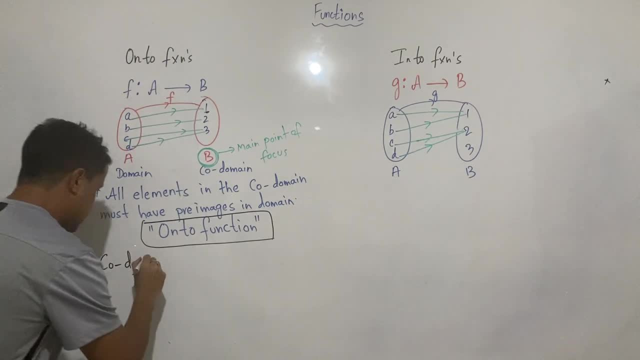 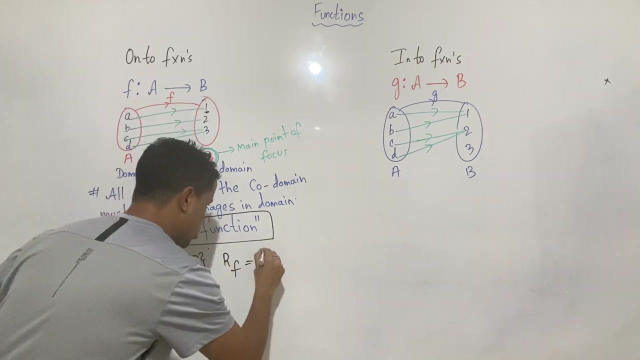 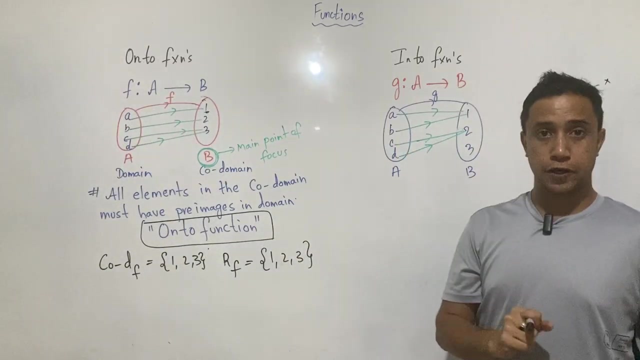 code domain of this function, f it is. it is. what is it? it's one, two, three. okay, one, two, three. and if you look at the range of this function, the range means the images, images. so it's again the same: one, two, three. so when your function is an onto function, if that happens, it. 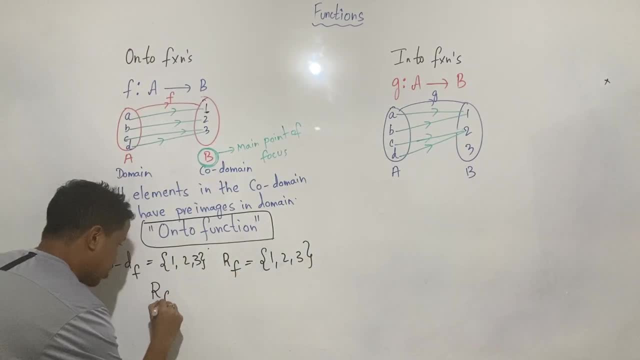 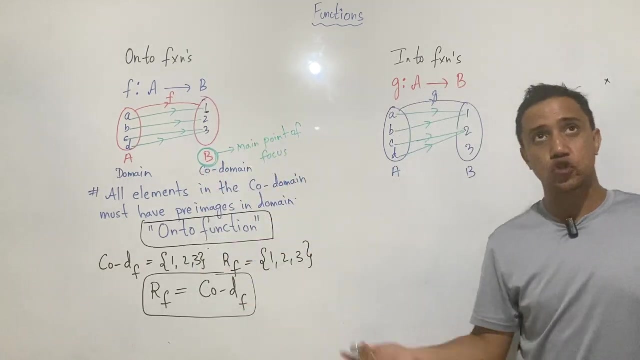 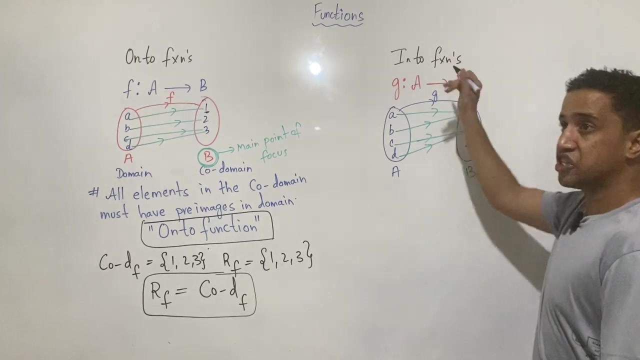 means your range, range of the function. it's going to be same as co domain of the function. I hope you got my point, okay, why? because then range is going to be equal to code domain. only then your function is going to be the onto function. now come to the next type, which is into function. now, when your function is 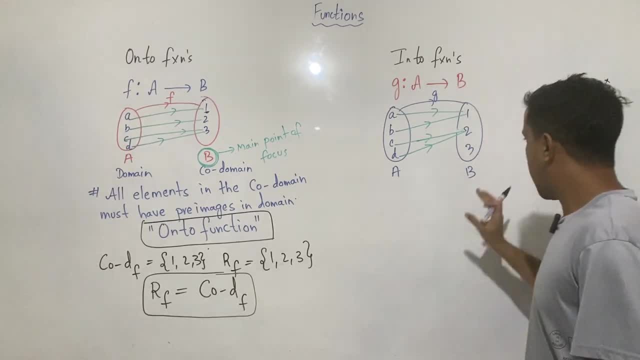 going to be into. okay, now, look again at the, uh, the the. look at the code domain. this is code domain. okay, so this is our main point of focus, of focus. okay, now one has a pre-image. does one have a pre-image? yes, two pre-images, a and b, to have image pre-image. sorry, yes, two. 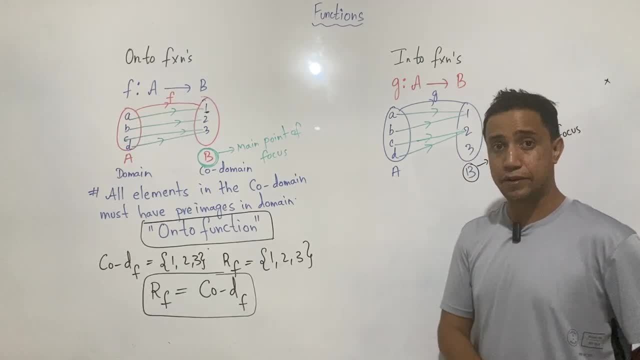 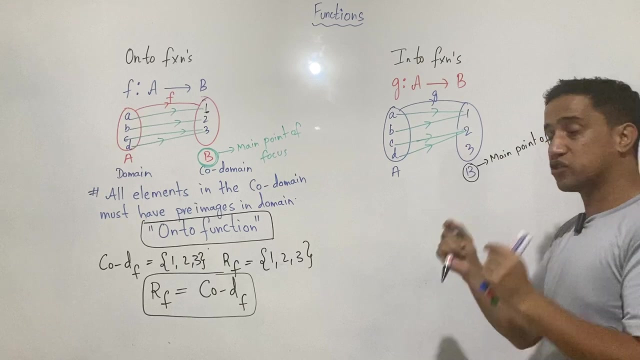 pre-images c and d. what about three? three doesn't have any pre-image. what does it mean? it means there is no element in a which is linked to or related to three. right, so this is going to be your. your into function, because there is- at least, there must be, at least one element. 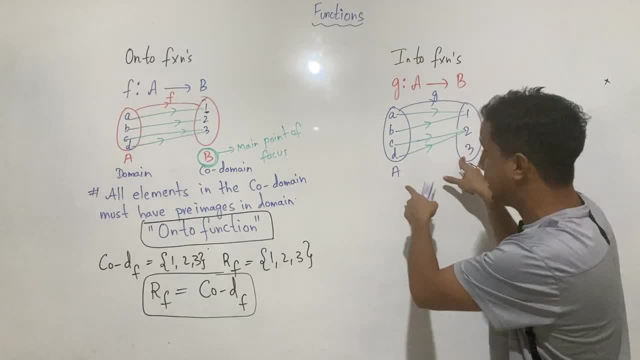 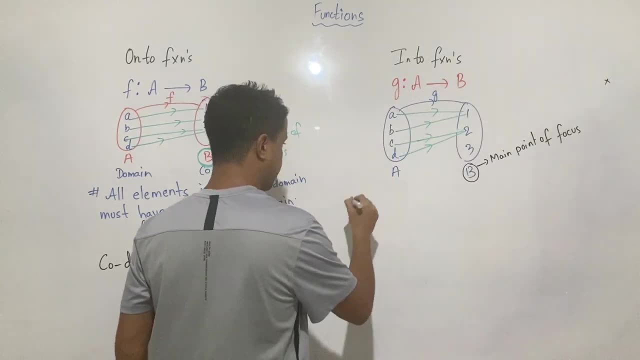 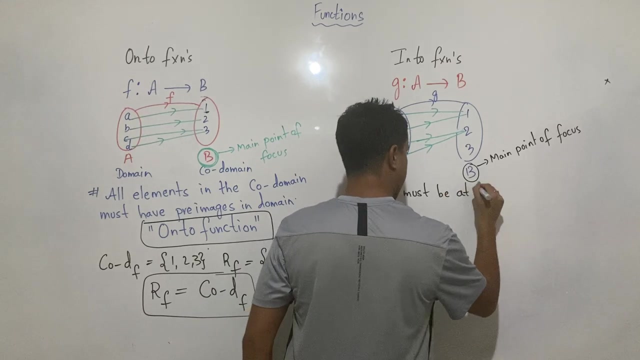 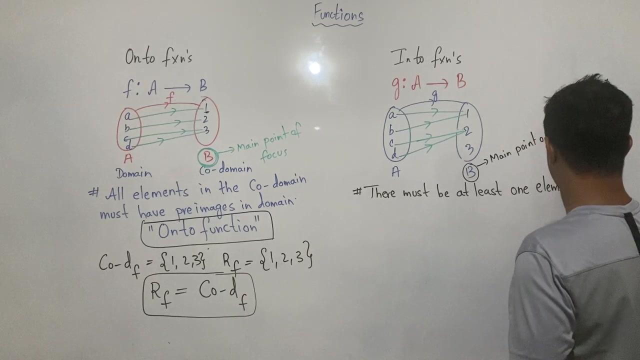 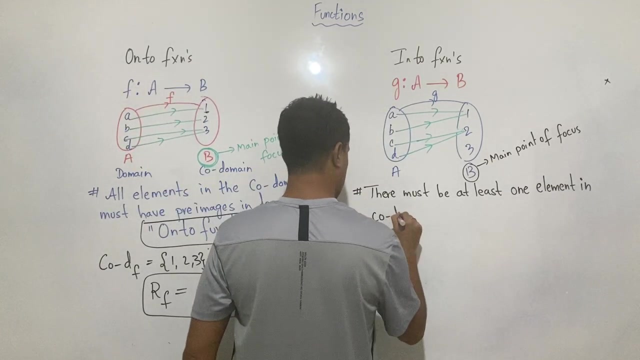 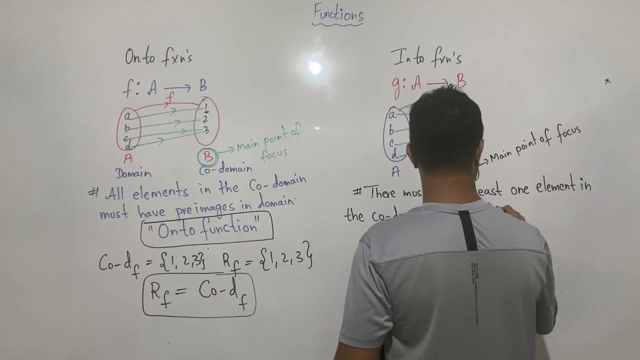 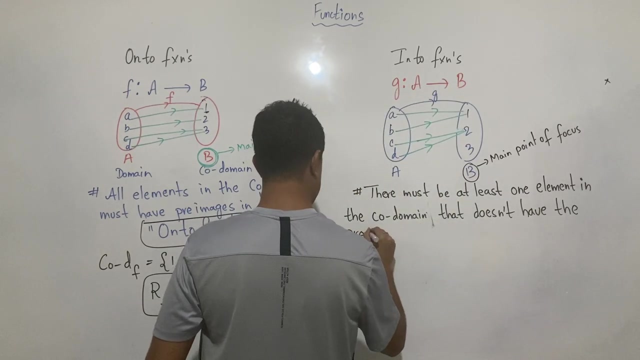 in your code domain which doesn't have pre-image in a. only then your function is going to be the into function. okay, so here I can write: there must be at least at least list one element in uh, in the code domain, code domain that that doesn't have the pre-image pre-image. okay, so this is going to be the. 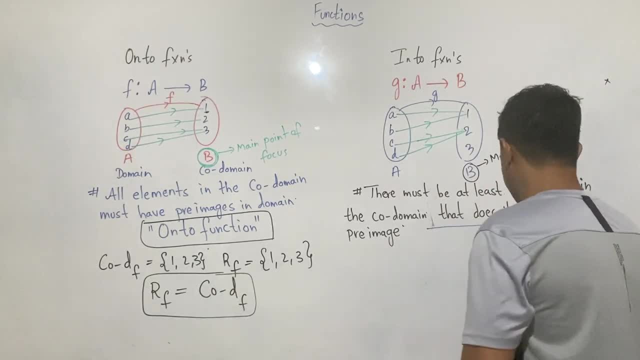 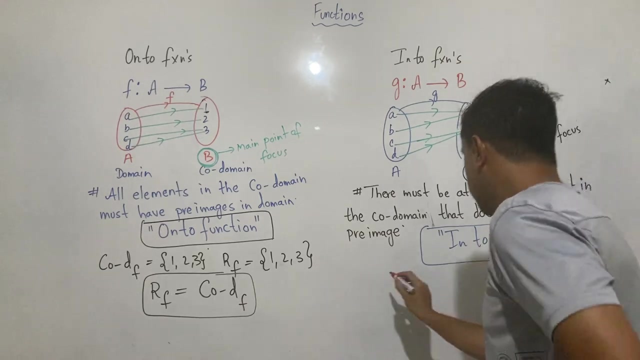 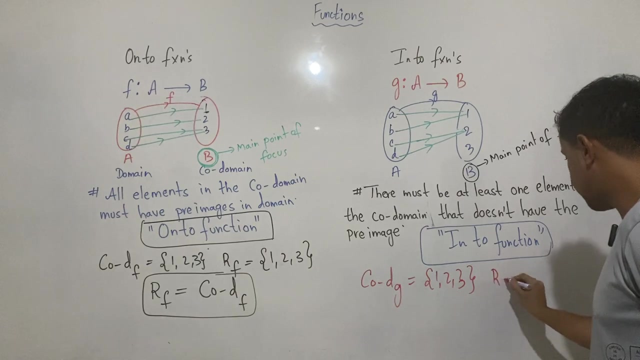 definition of your your into function. okay, so this is going to be your in two function. okay, into function. now, if you look at this, the, if you look at this here, your code domain, your code domain of g is, uh, what it is? one, two, three, one, two, three, one, two, three. and the range, range it's. 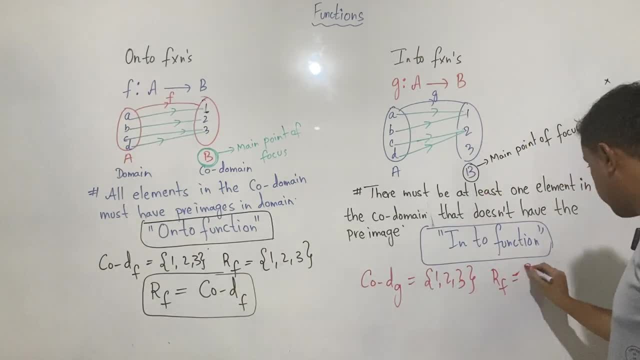 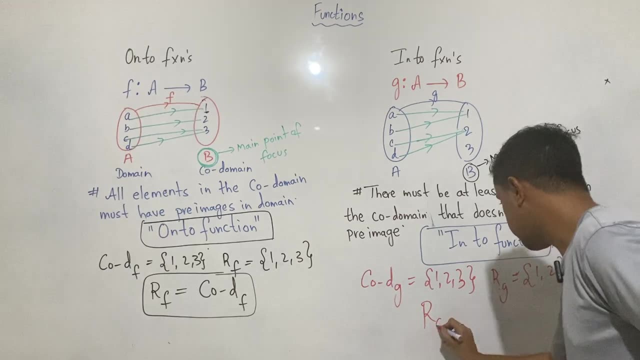 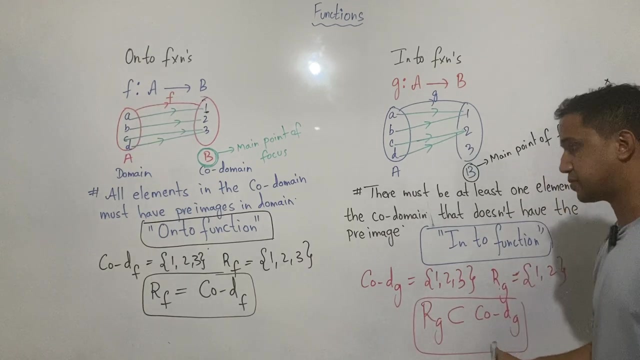 going to be. range means images. so, uh, it's going to be one and two. so you can see here, here, your and two. so you can see here, here, your range is going to be the subset of code domain. your range is going to be the subset of code domain. here your range is similar to code domain. 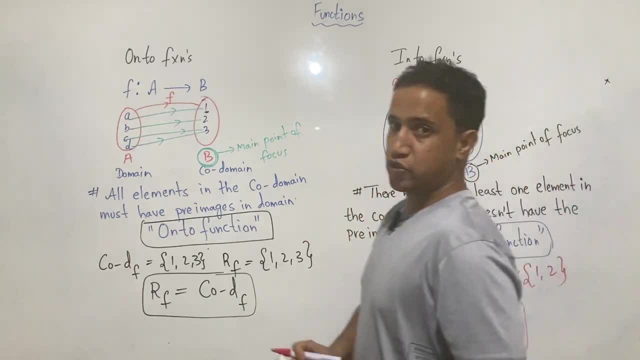 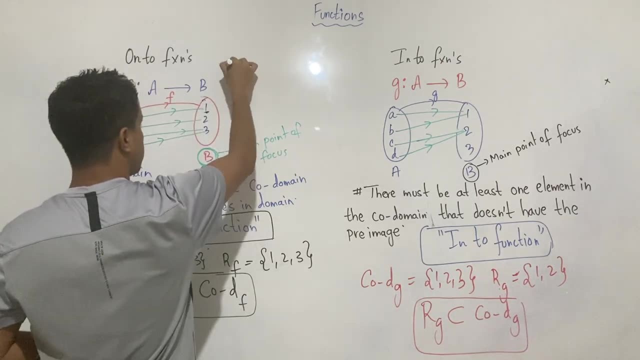 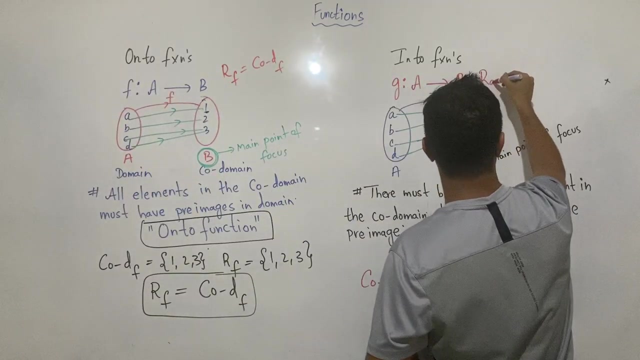 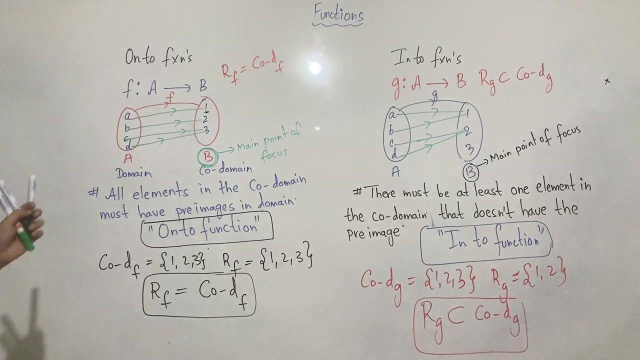 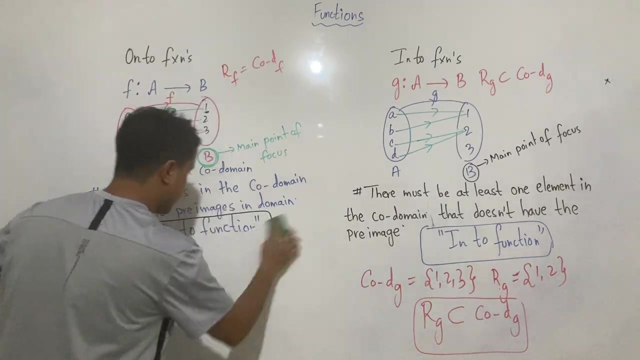 okay, so that's the difference between your onto functions and your into functions. I hope things are clear. here your range is same as code domain and here your range is the subset of code. okay, so I hope it is clear to you. okay, now let's take- uh, take an example for more clarity. 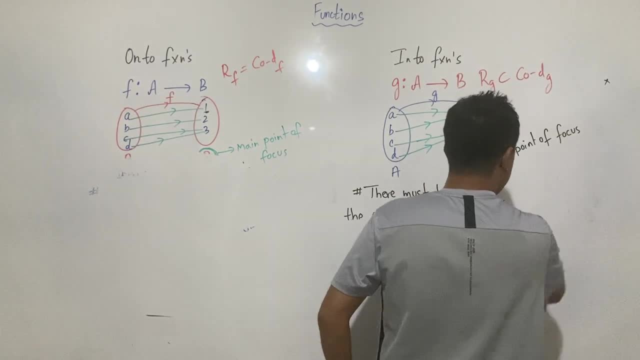 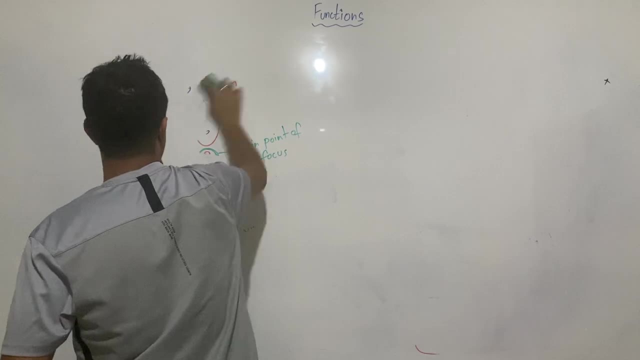 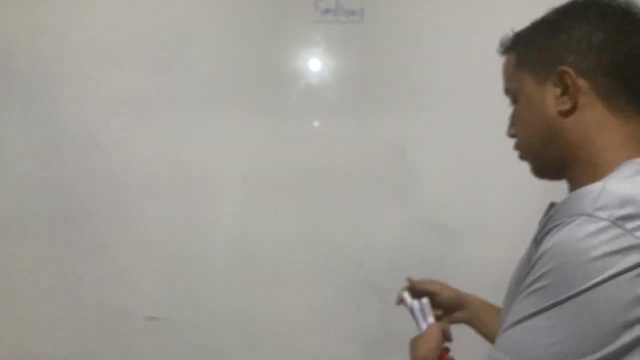 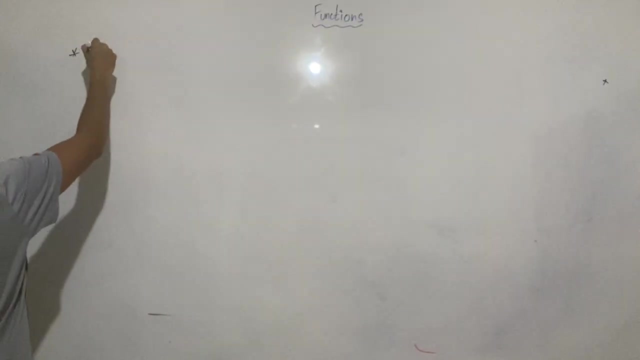 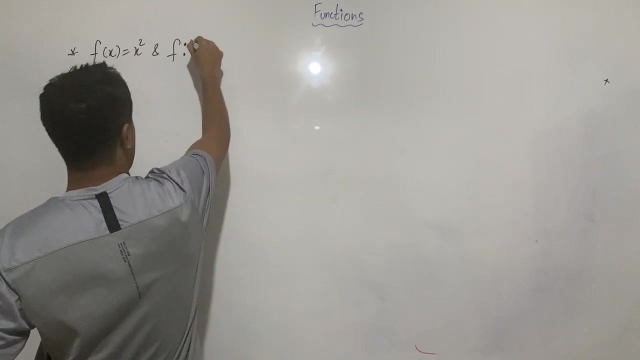 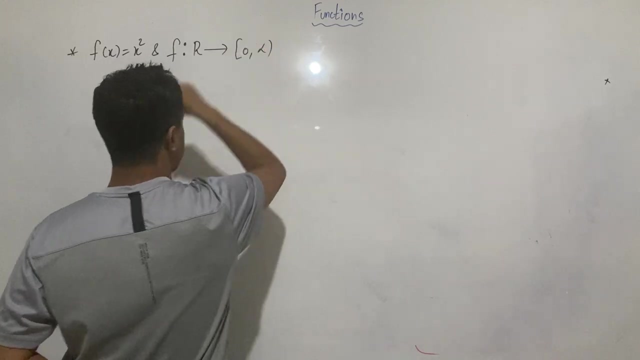 okay, I have uh. I have two functions here. let's take an example: here I have a function, fx equal to x square, and uh. this is defined from uh and your f is a function. it's defined from uh. r to zero, to infinity. okay, and here your fx is a same function. 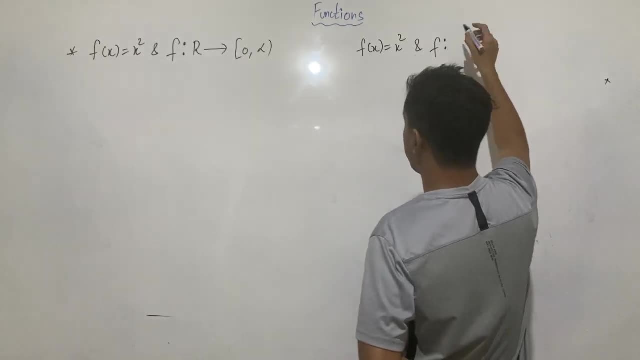 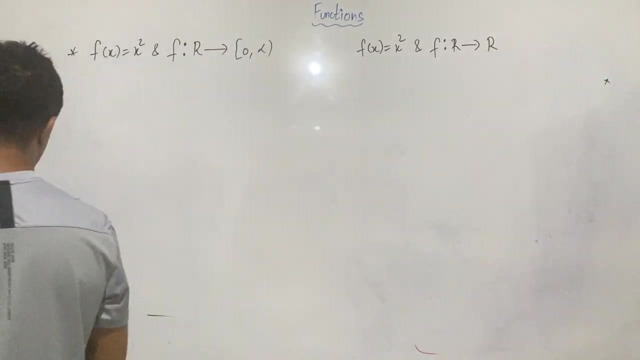 of x square and it is defined from, from our to our. okay, so we have to show which one is on to and which one is into. okay, now see here, uh, sorry, so what we can do here is: uh, what is the given function? given function, is our fx equal to fx equal two, fx equal two? so so we will want, we will want, go to into uh, so there's uh, there's four, uh, three different types of data, so the core numbers and, of course, the custody of the family, in terms of which color is important. we don't have. 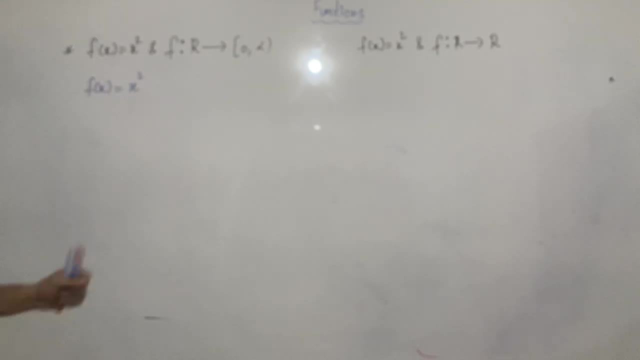 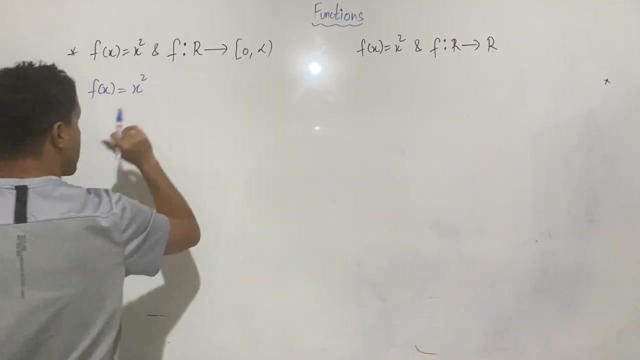 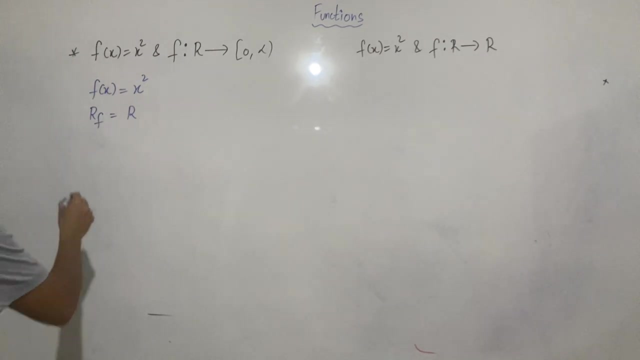 f, x equal to x square, And if you look at this mathematical form of function, you can say that the co-domain is given to us. Now see here: range of this function is all real numbers And co-domain of this function it's going to be in this interval, 0, closed. 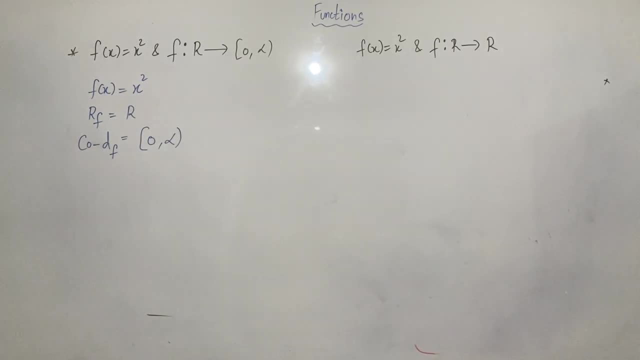 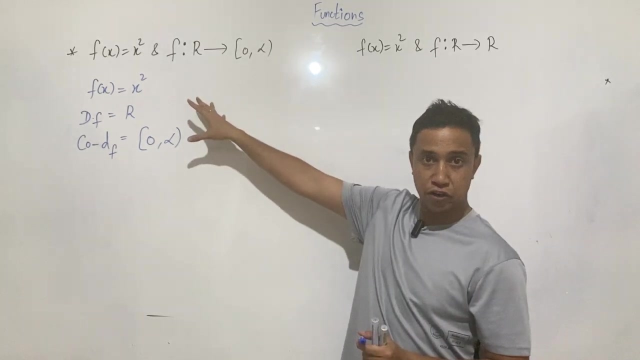 interval 0 to infinity. okay, Now, this is the domain. sorry, not range. okay, Now we don't know if this function is onto or into, so we have to find out the range, right? If we know the range, then we can deduce whether this function is going to be onto or into. 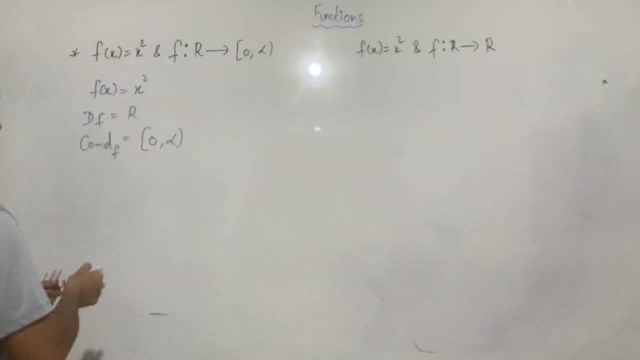 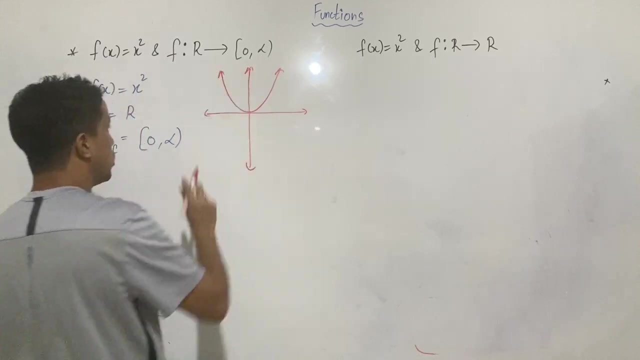 okay Now, if I look at the graph of this function, y equal to x square, because this is quadratic, right? So I'm going to get a parabola, right. So here you can see that the y- y is always going. 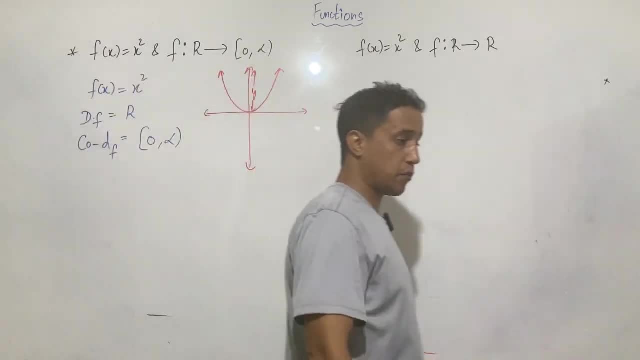 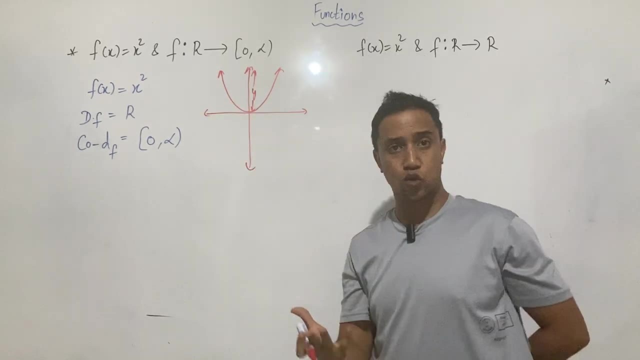 to be positive. right, Y is always going to be positive. It's going to be greater than equal to 0.. Why Why? Why, Because at origin, y is going to be 0, and on both sides of x-axis you put any value. 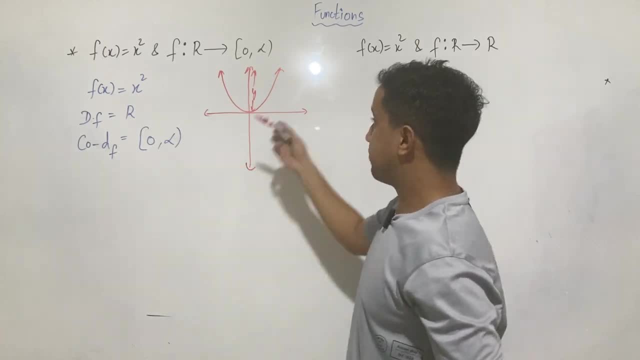 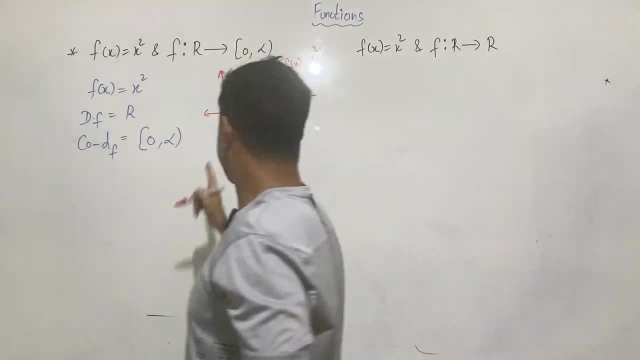 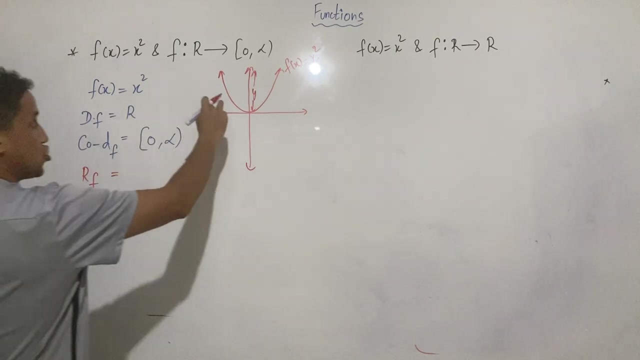 then y will always give you the positive values, because the function is: fx equals to x square. okay, So I can say from here the range of this function. it's going to be what It's going to be. it's going to be 0 to 0, to infinity. 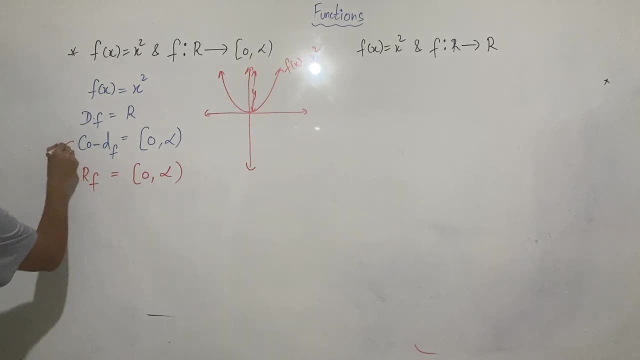 Right Now, from here, I can say that my range is same as my codomain right. So if this is the case, then I know my function is going to be onto. So here f f is onto function. 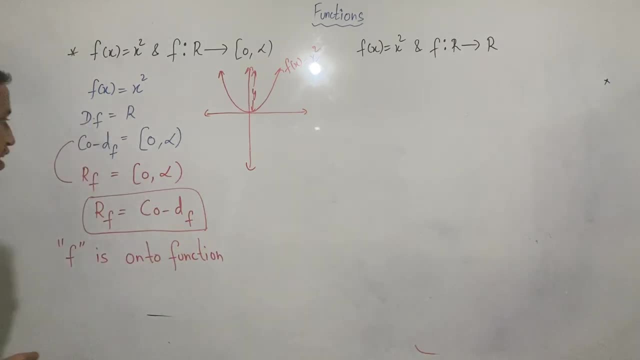 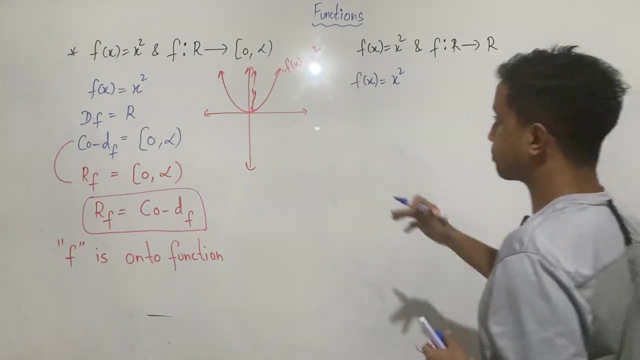 I hope you understand it Why? Because codomain And range, both are same. Okay, Now come here. Here the function is: fx equals to x, square right, And here the domain domain, here is domain, Which is domain, Domain is. 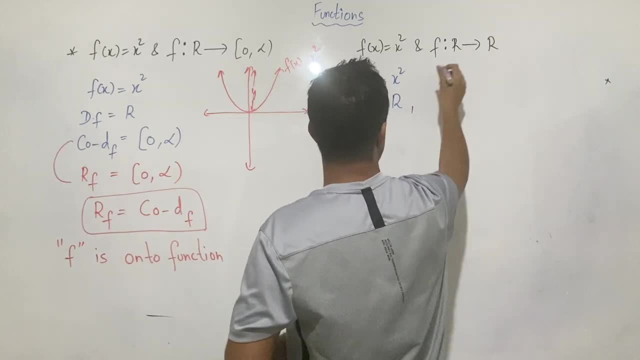 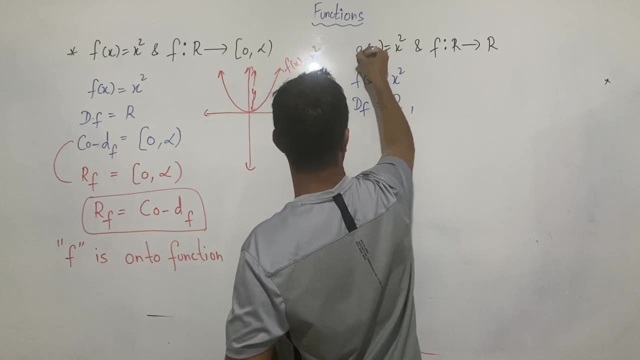 this Domain means all real numbers And here the range of this function, f. here we can say this is g, okay For, For differentiating it with this function. So d of g is r And codomain, codomain of. 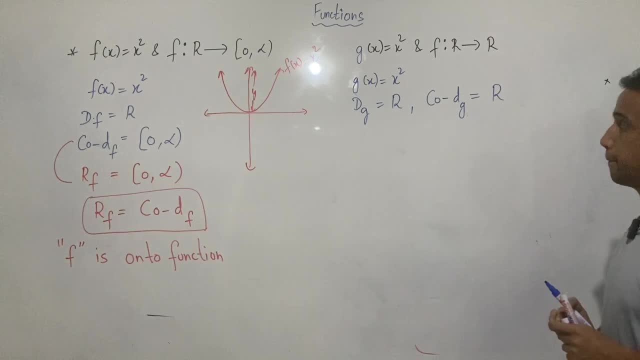 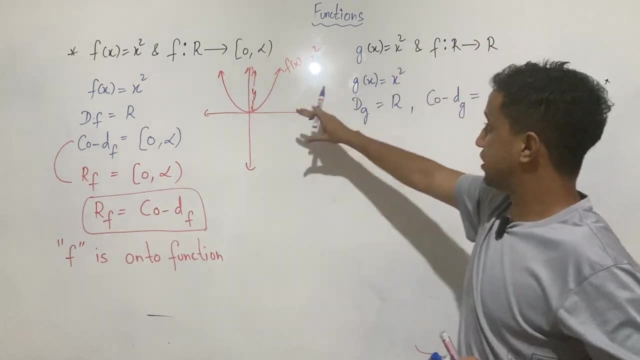 this function g. it is also r Right, Because codomain is r, domain is r. Now we know that the range of this function it's always going to stay 0 and positive. The minimum value is going to be 0. 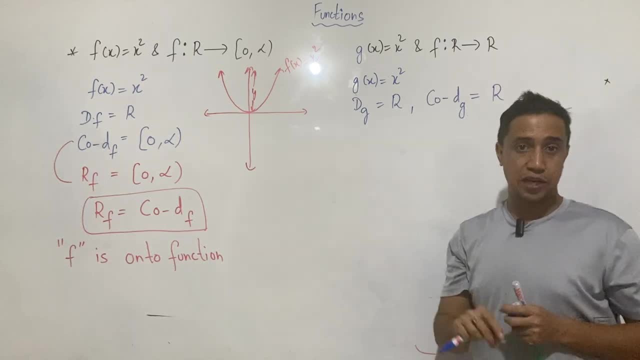 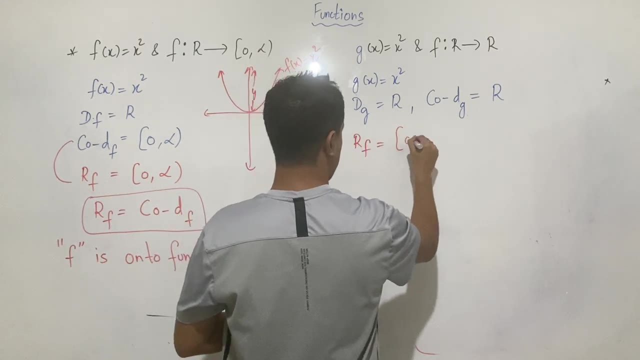 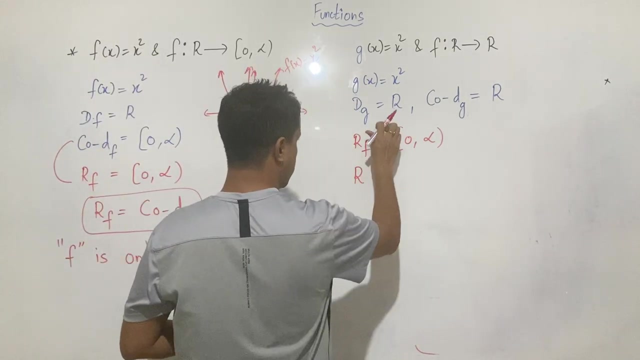 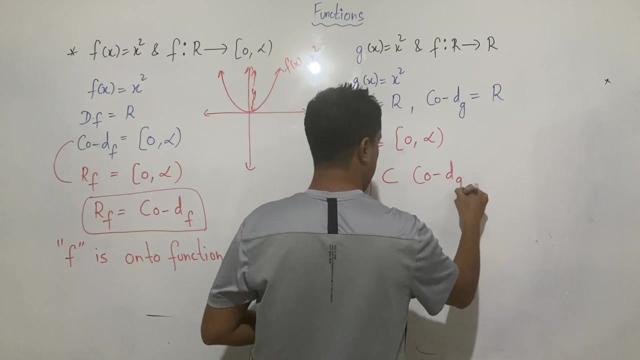 And other than that, it can take any positive values. Okay, So here I can say that the range it's going to be 0 to infinity. Okay, So, from here what I can say, that my range, range of g, this function g, it's going to be subset of codomain, right? So therefore? 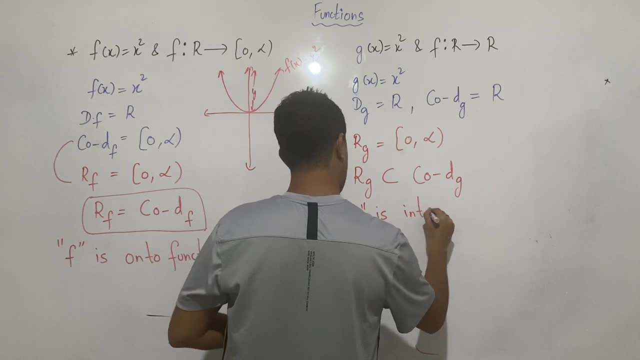 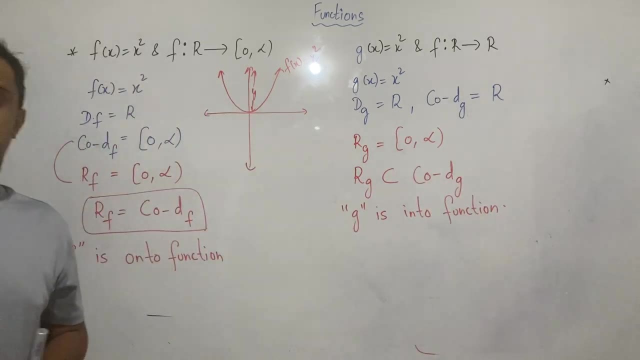 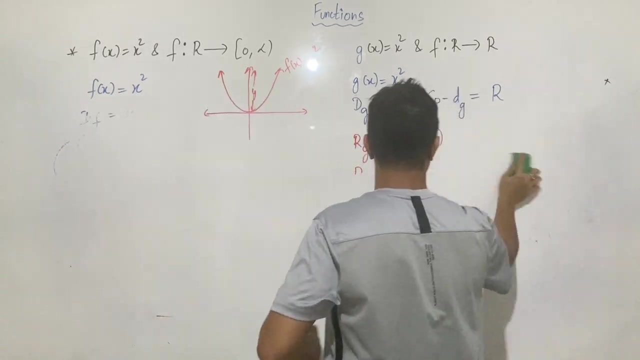 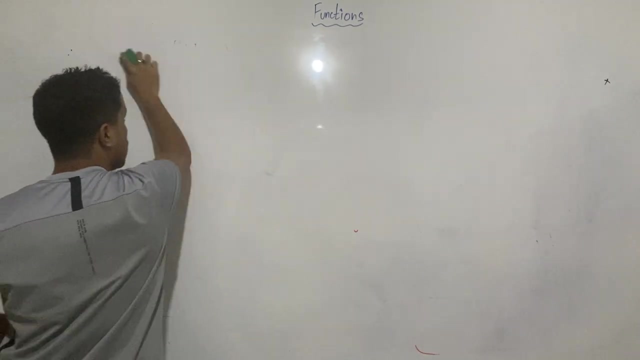 g is into function. I hope things are clear to you All right Now. if this is clear, then just take note of some more points. Take notes of some more points, Okay, In the previous session, in the previous session, when we had our previous session. 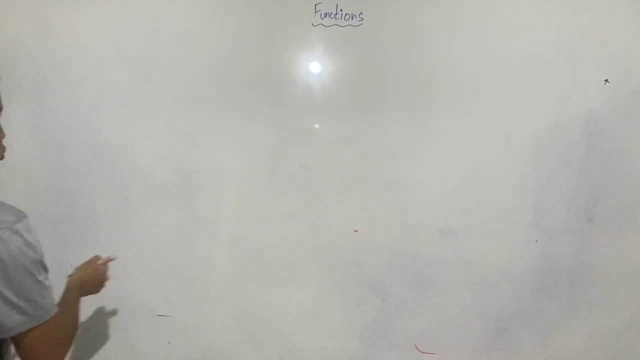 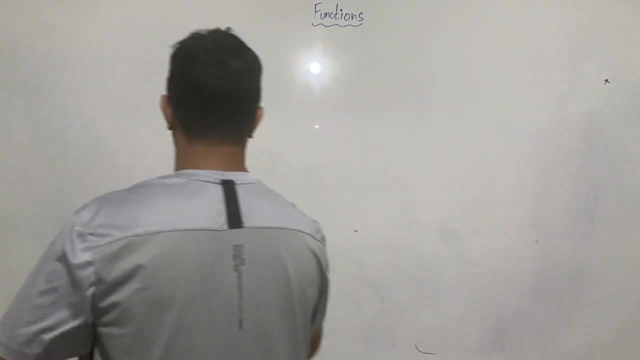 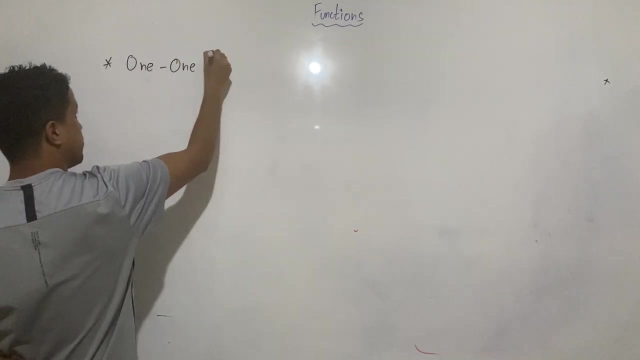 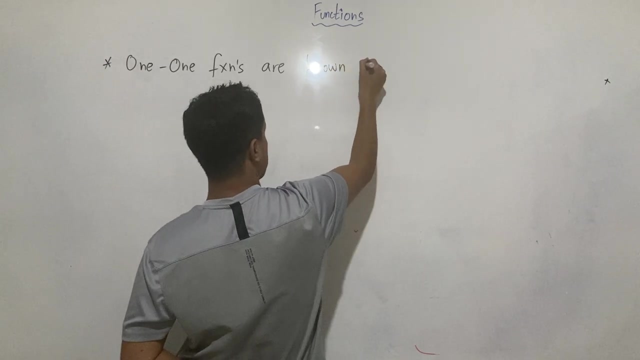 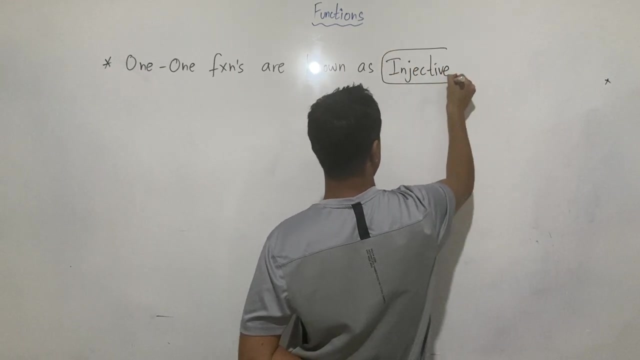 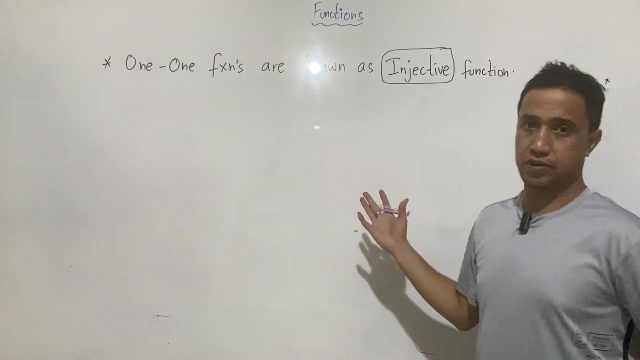 then there was one thing that I have told you, And what was that? I have said that. I have said that 1, 1 functions are called, are known as as injective functions. right Now, many one function doesn't have a such name. OK, 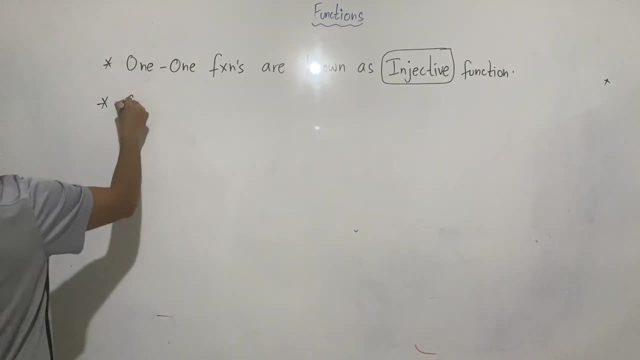 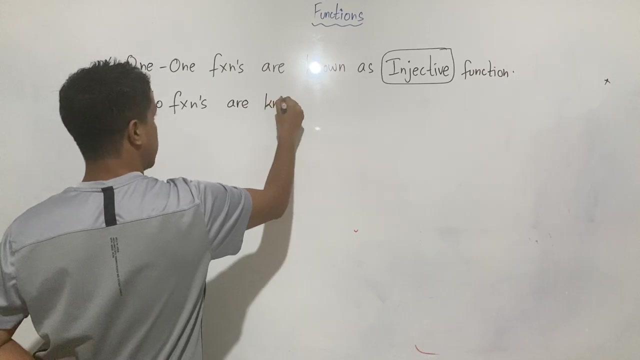 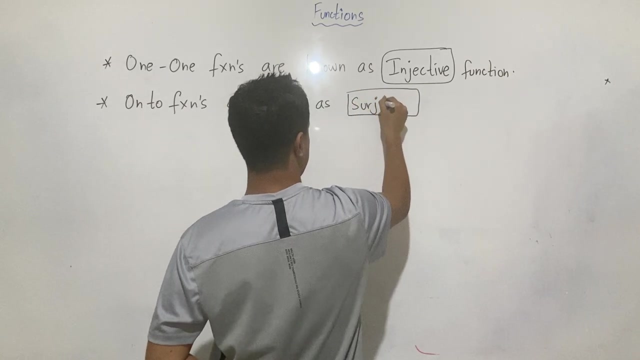 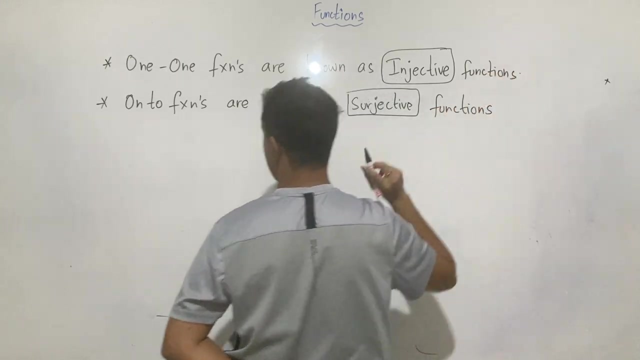 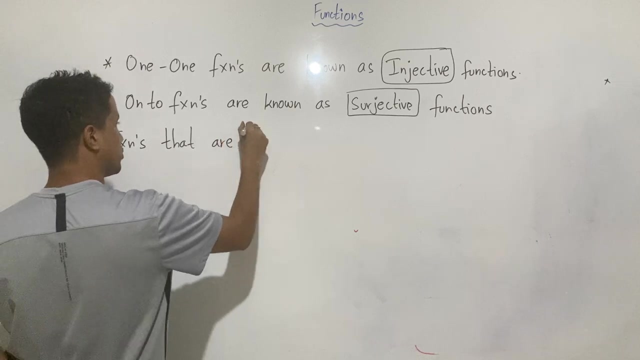 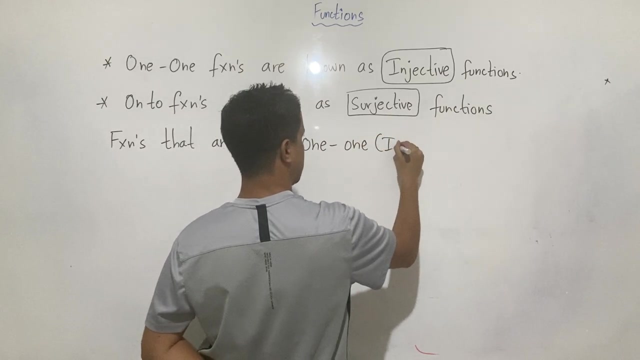 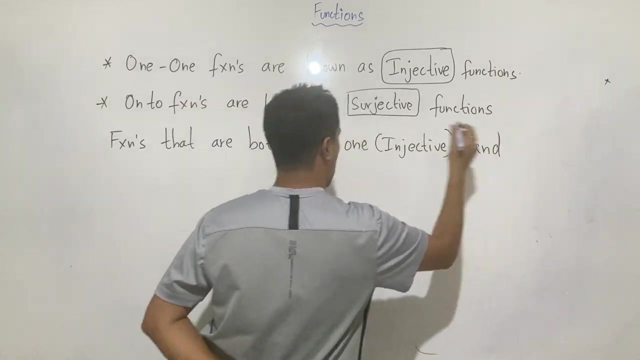 Similar to this. we have this: onto functions are also functions are known as known as surjective functions. OK, Surjective, surjective functions. functions Now, functions that are both both one one. one one means injective, injective and and onto, and onto means surjective. 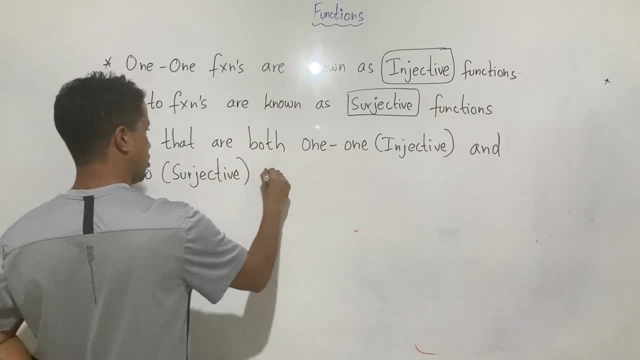 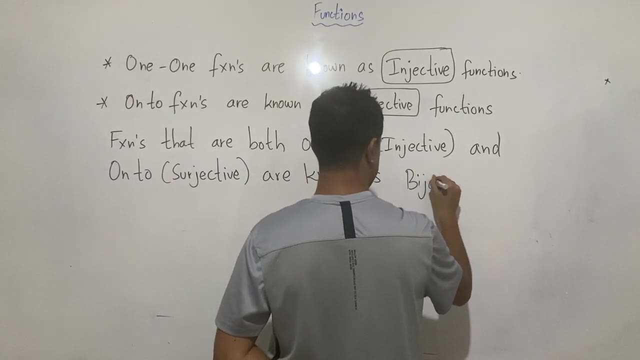 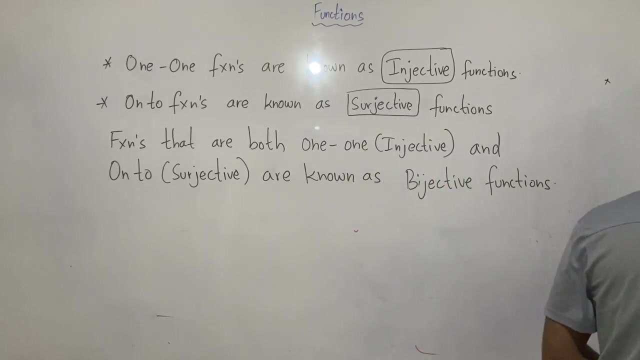 are are known as bijective- OK. Bijective functions- OK. This is important. Just keep this thing in your mind: that if your function is both injective and surjective, then it is known by the name bijective function. OK. 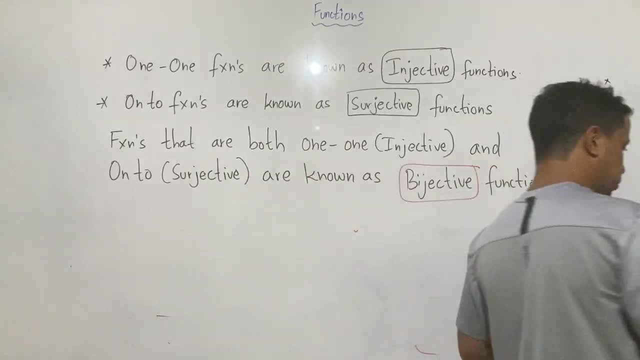 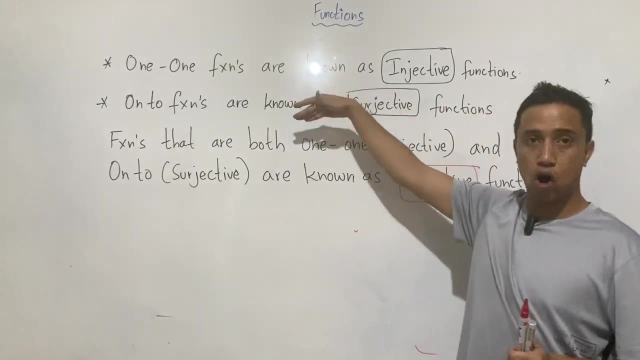 So let's see what it means. OK, I hope this is clear. Simple: One one are injective, onto are surjective. So functions that are both one one and onto they are bijective. OK, Now let's see. 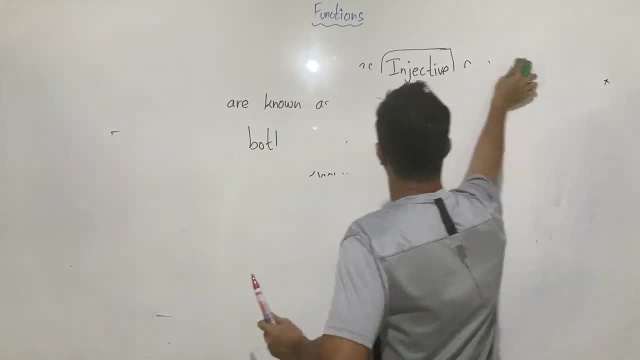 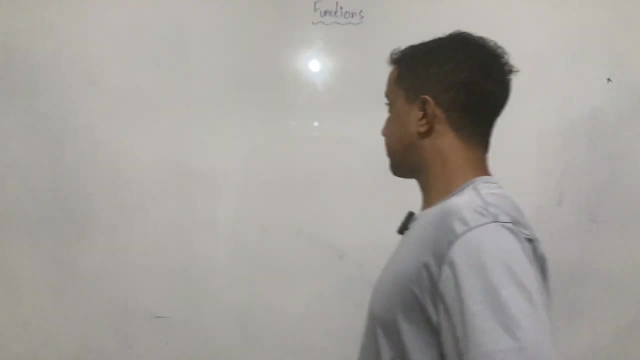 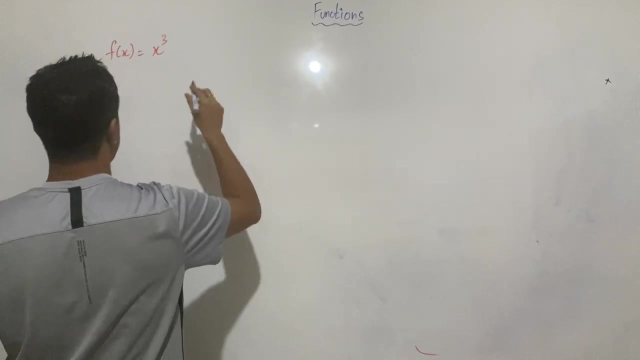 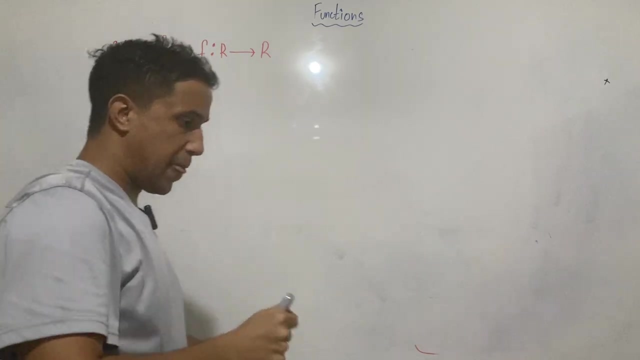 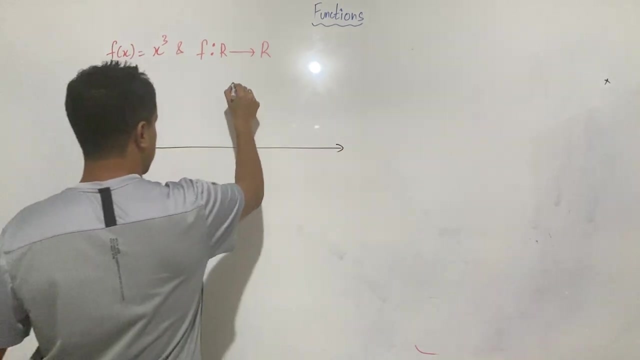 Let's take one function fx equal to xq. OK, This is a function fx, fx equal to xq- OK, And your f is defined from r to r- OK, Now see here if you make the curve of xq. 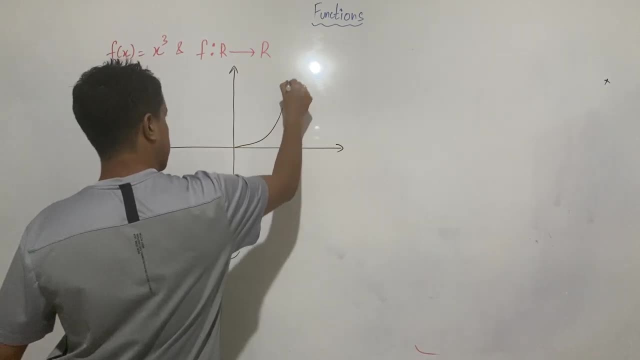 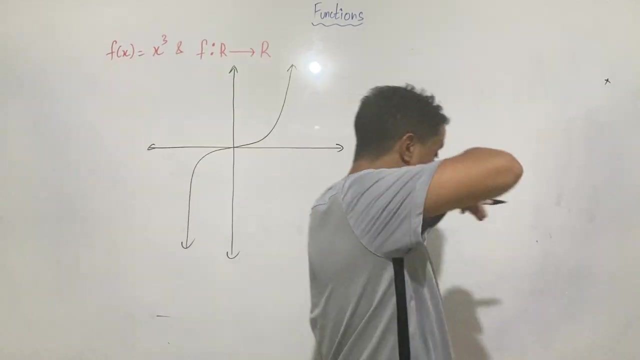 then it's going to be: you know xq right It's going to be: you know xq right to be like. then it's going to be like this: okay, and if you will draw any horizontal line on this, 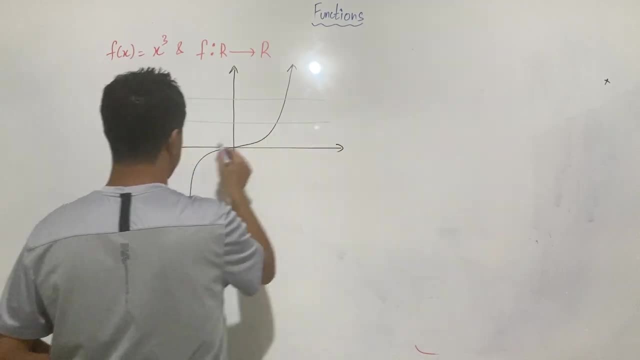 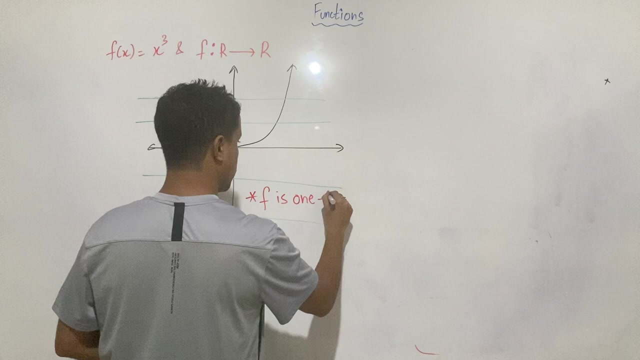 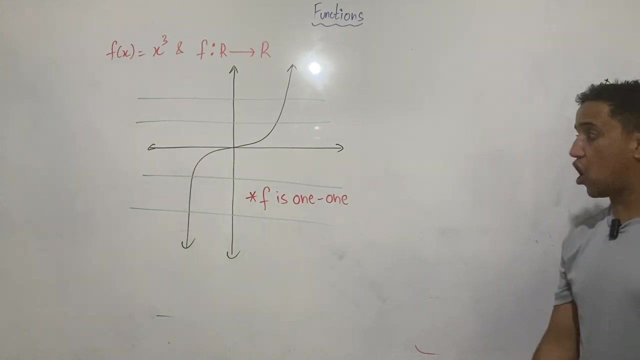 curve, then it won't cut the, it won't pass through the curve more than once, which means that this is here, this is here. f is one one, right, one one. now let's say, let's see that if it is also uh one, sorry onto function. so here we have f that goes from r to r, defined from r to r. so 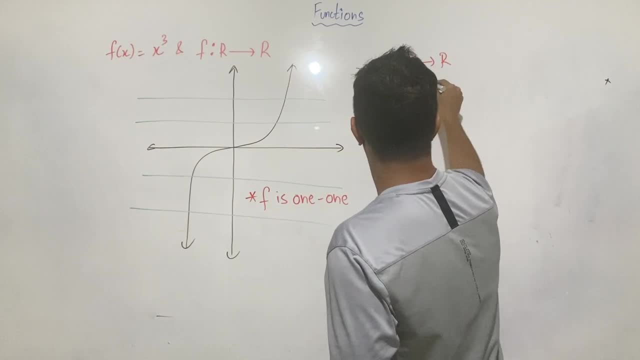 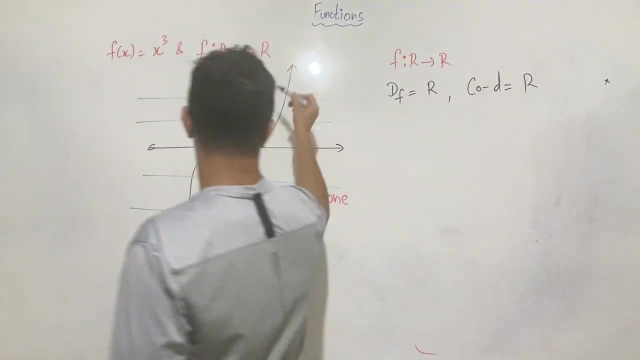 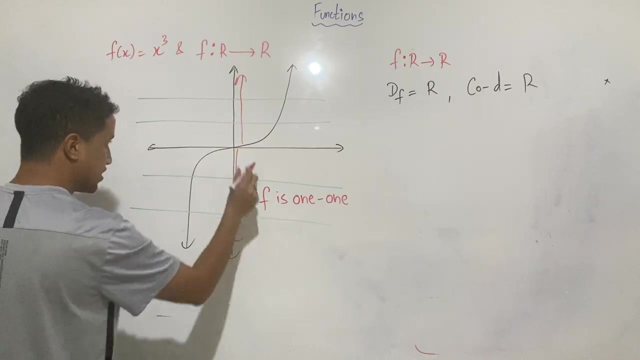 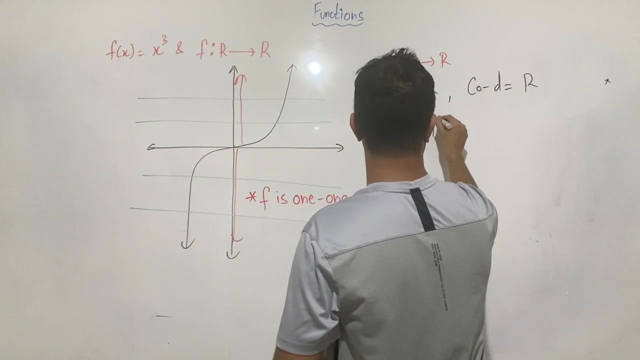 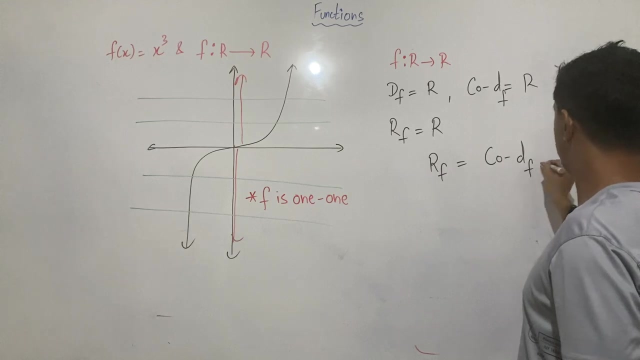 here domain it's r and your code domain it's also r. if you look at the range of this function now see: here your y can take positive values, your y can take negative values. here it is zero, so it means that your range of this function is also r. now our range here it is similar to our codomain, right codomain, so which means that. 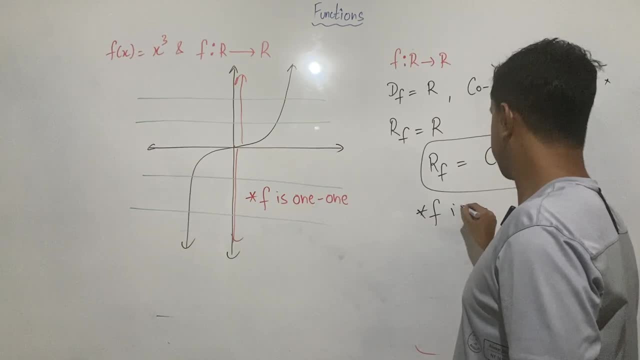 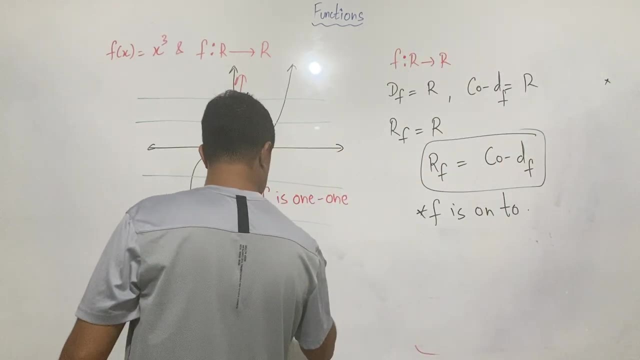 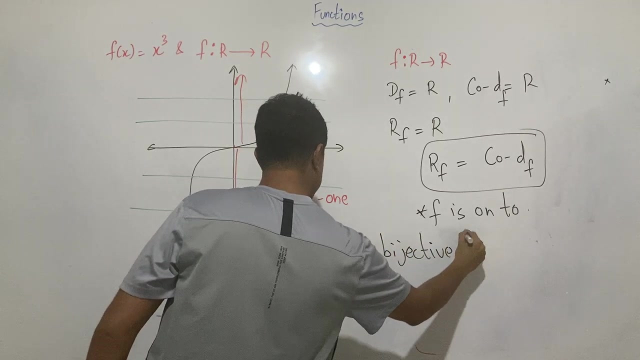 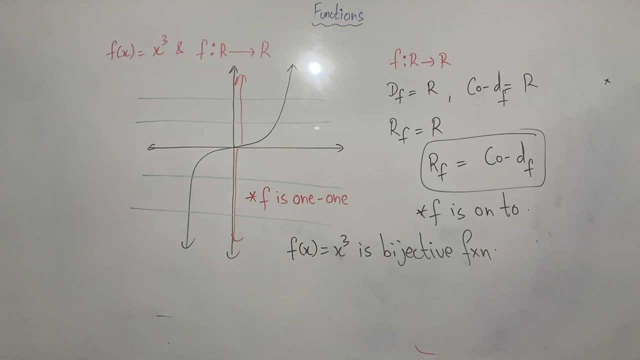 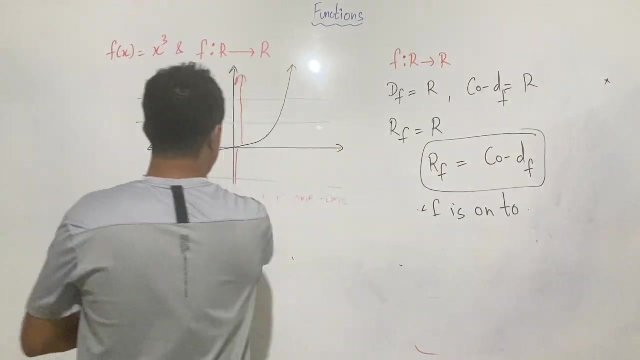 this function is f, f is f is on two, on two, okay, so f is one, one, f is on two. so f, x equal to x cube is bijective, bijective function. i hope it made sense to you, so just have a look. okay, so now let's do some question. 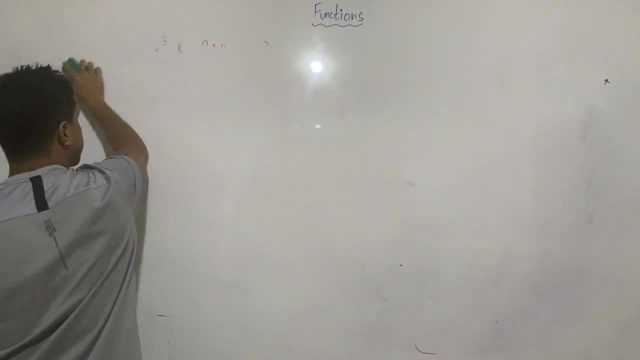 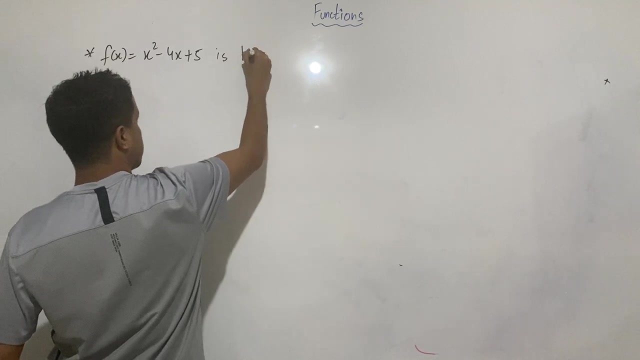 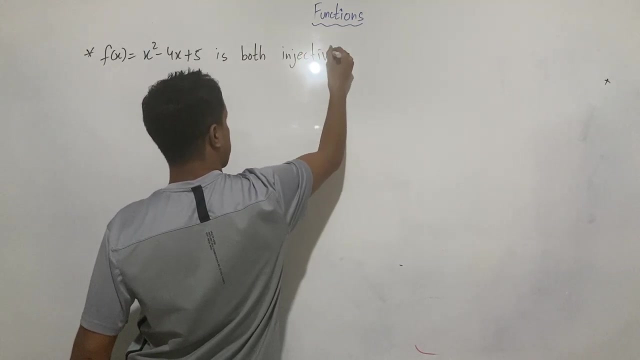 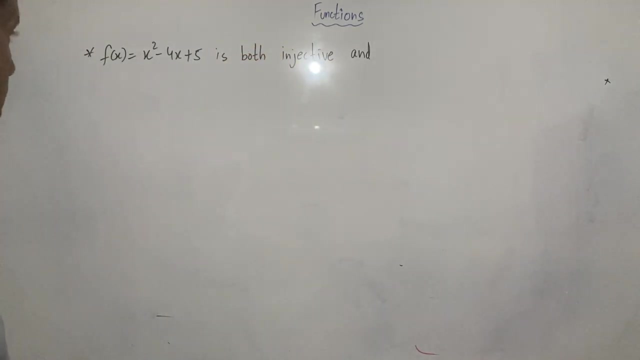 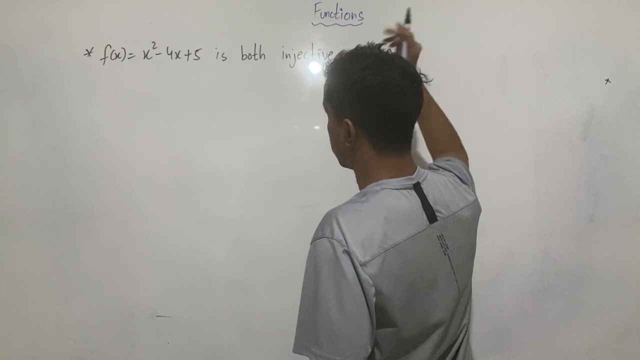 so write down the first question. so the first question is that your function fx equals to x here. minus 4x plus 5, uh is both, both, uh is both injective and uh, it is both injective and uh, onto uh and on two. okay, and this function is defined uh, this function. 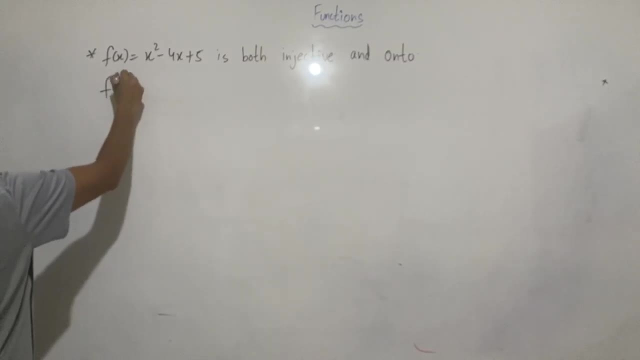 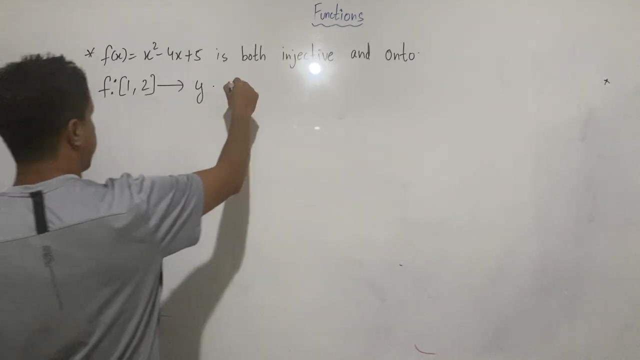 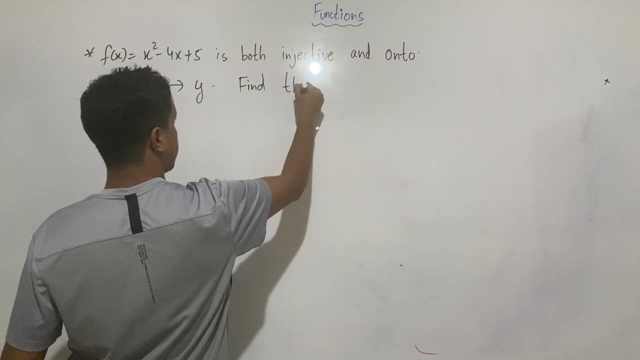 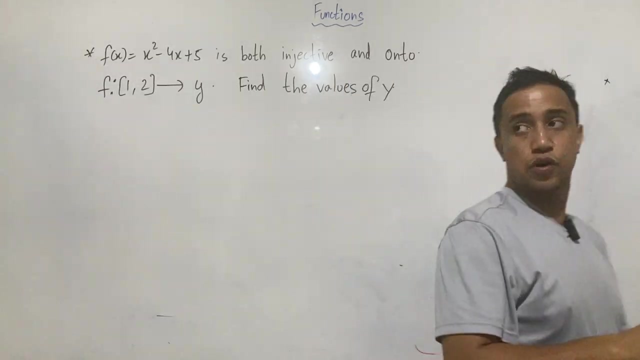 is defined from uh. it is defined from this interval: one, two, two, uh, two, y. okay, so you have to find, find, find the values of y, you find the values of y, or in other words, you can find the values of y, y, or, in other words, uh. you need to find the uh, the codomain right. so now see here, this is the given. 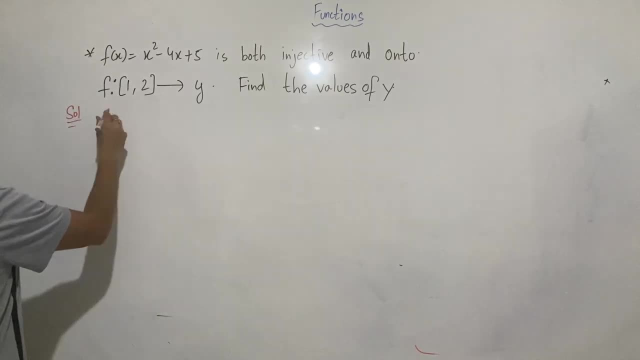 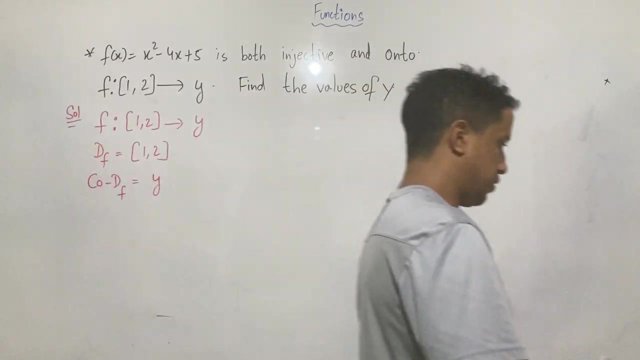 function: uh, solution. okay, so the given function is defined as one, two, two, two, y. so domain of this function it is one to two and range, sorry, code domain. code domain of this function: it is y. okay, now, what type of function is it? now, let's see this. is this is what this is, quadratic, right? uh, f, x. 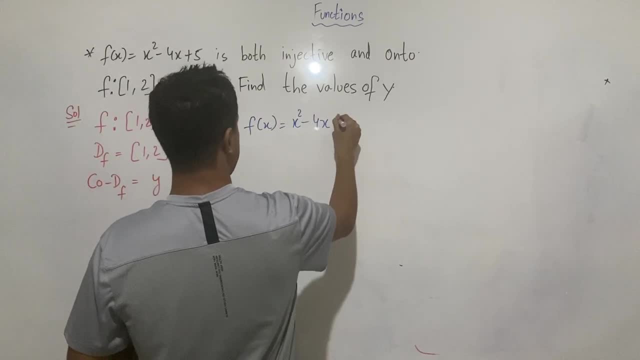 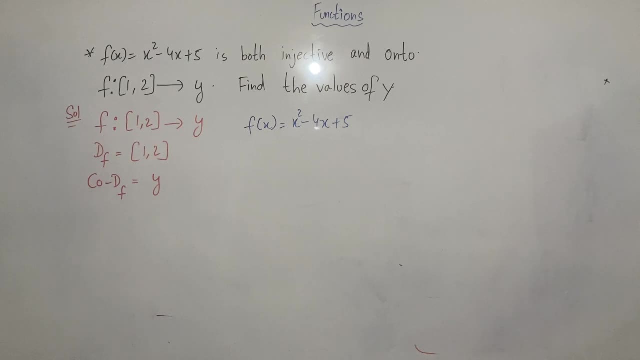 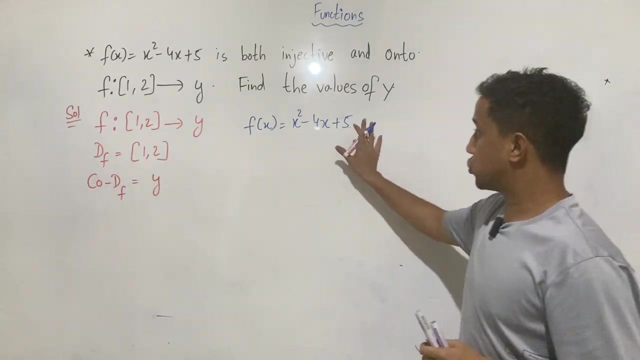 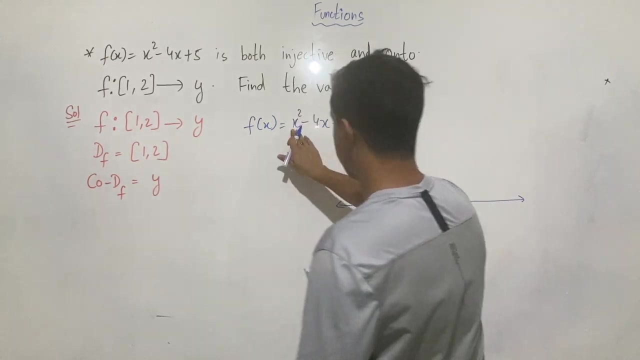 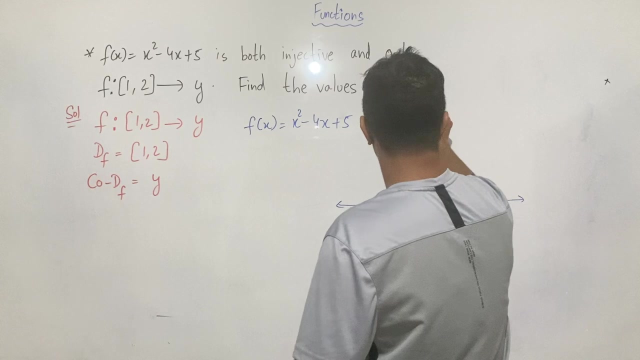 equal to x square minus 4, x plus five. all right, this is quadratic. okay now, uh, this is quadratic. uh, so i know that if i want to sketch the graph for this quadratic, because this is positive, a is positive. a, x squared plus p, x plus c. it is of the type right, so a is positive. it means i am just going to get. 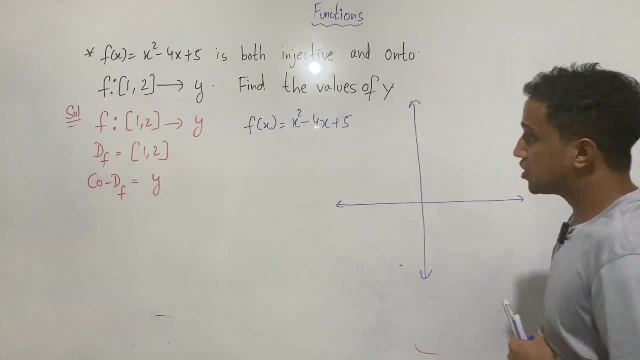 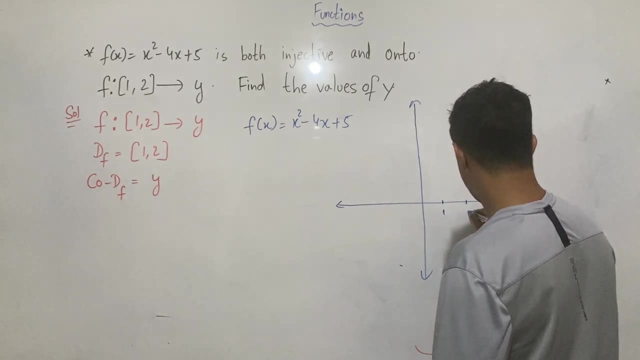 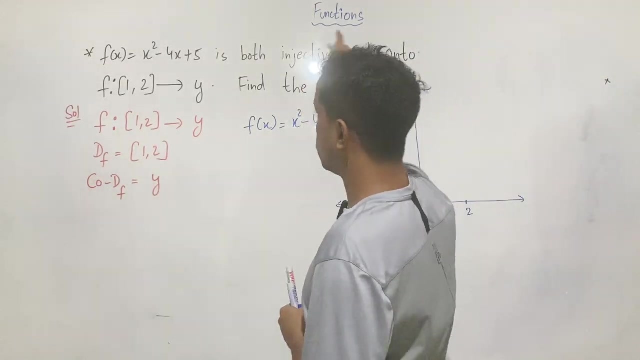 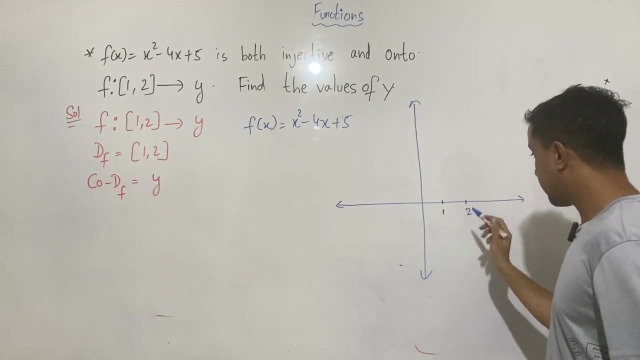 the upward parabola. upward parabola, but here my domain is one to two, so here i have one and here i have two. okay, so this function is injective and onto in this domain, right, so this function is behaving as bijective in in this domain, only in this domain. okay now. 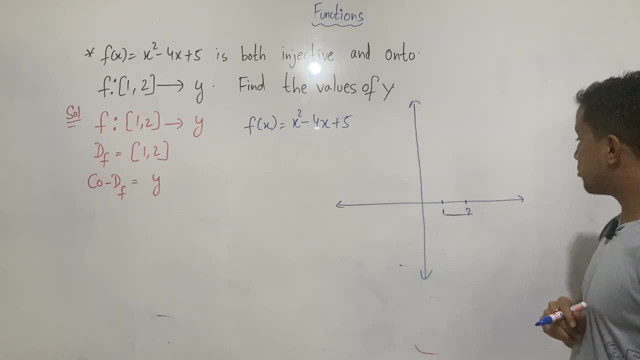 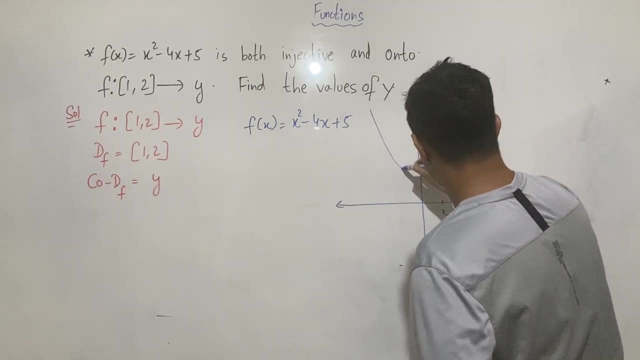 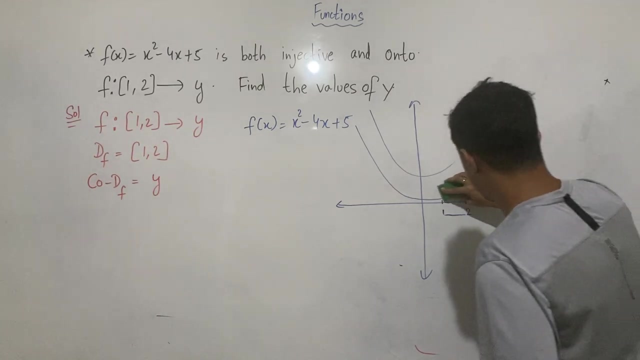 it's going to be. it's going to be the upward parabola, right so, uh, it could be of this type, it could be of this type, or it could be of this type, right so, uh. but because this function, here the domain, it is limited to the interval. okay, so here what possible things we can do. 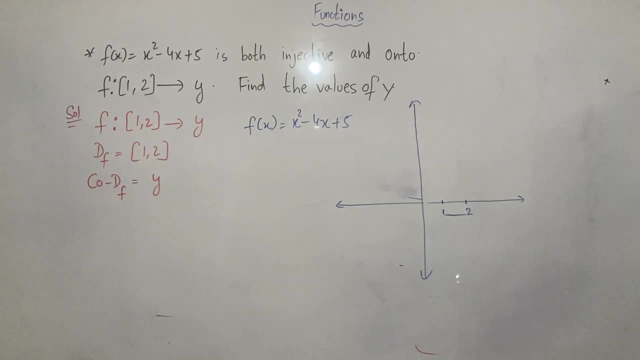 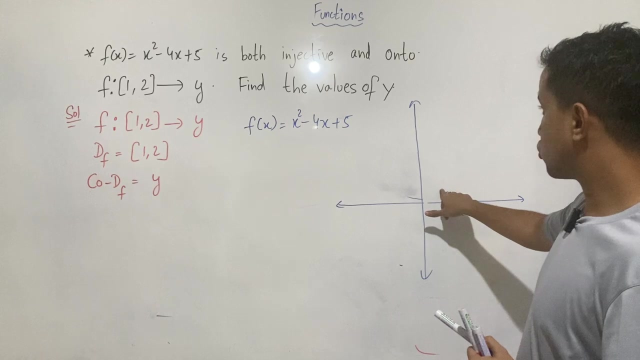 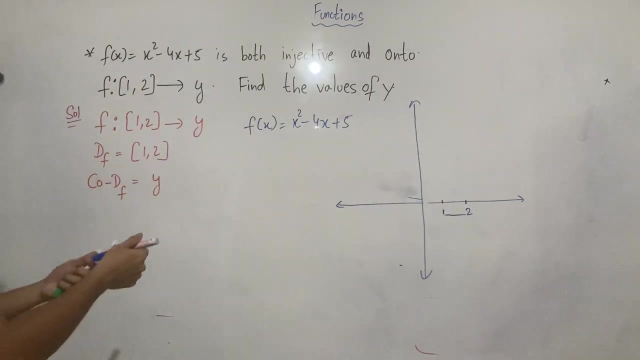 uh, what possible things we can do is that, uh, what's going to to be the value of this function at one? okay, so if, uh, i'm going to put here one, then it's going to be one. what about two, four, okay now, uh, if uh, what i can do here is that. 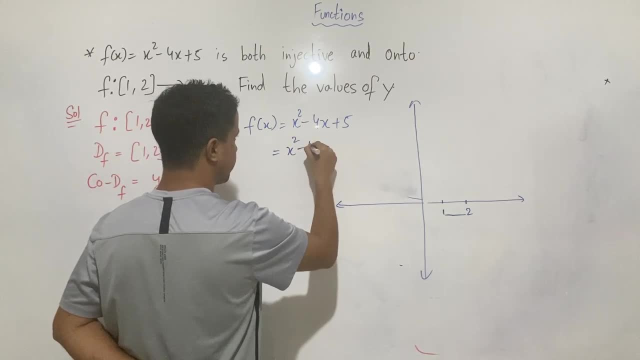 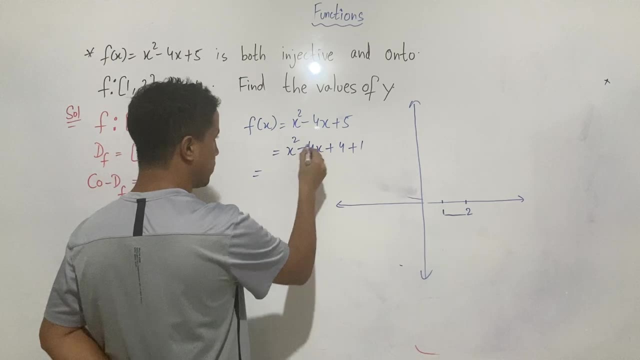 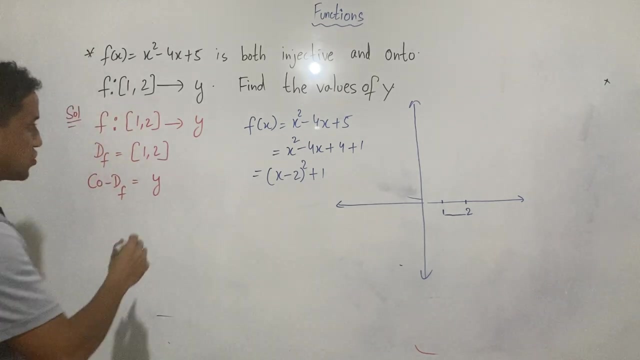 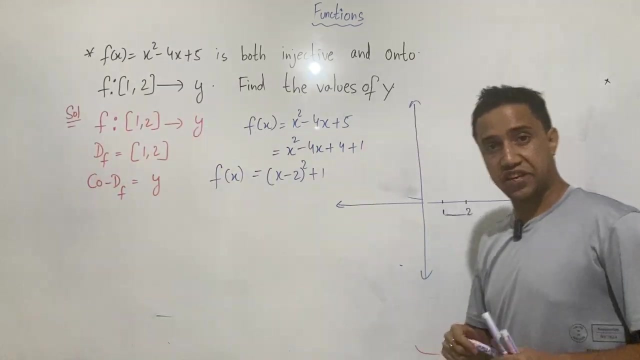 if i write it like this: x square minus 4x plus 4 plus 1, right, so it's going to be x minus 2 squared plus 1, if i am not wrong. right, so, because this is quadratic and i have just created few things here so that here i got something in the form that looks: 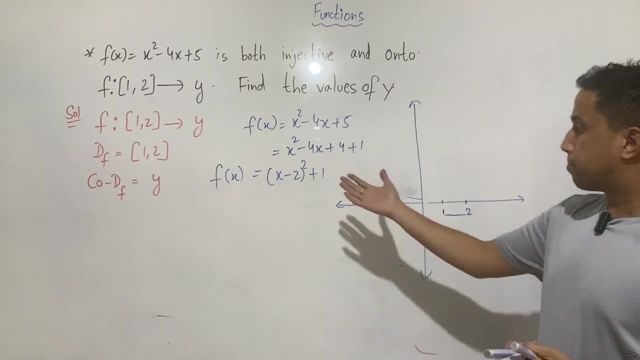 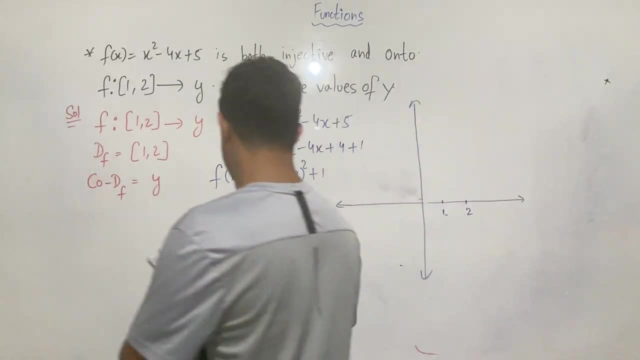 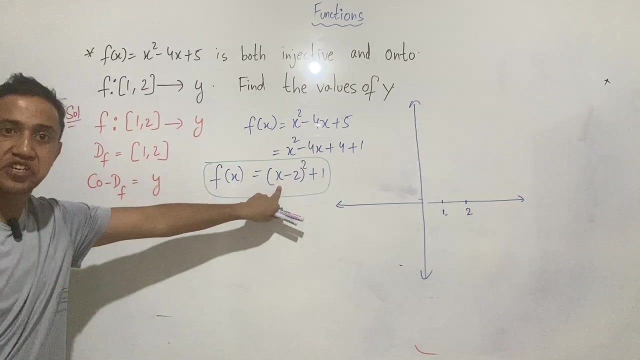 something in the form of factor. now, this is x minus 2, squared plus 1.. now, if you look at this, if you look at this, this function, now this function is going to have minimum value when this is going to be 0. right, this whole function value is going to be minimum when this thing is. 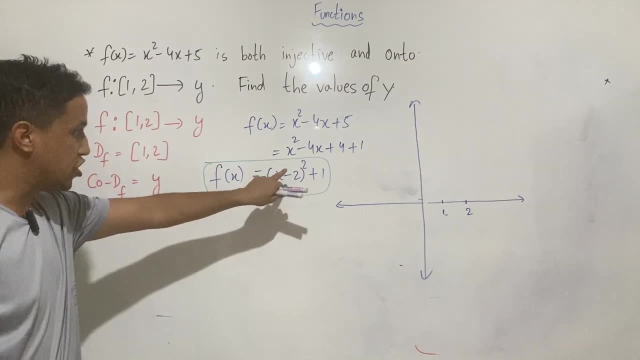 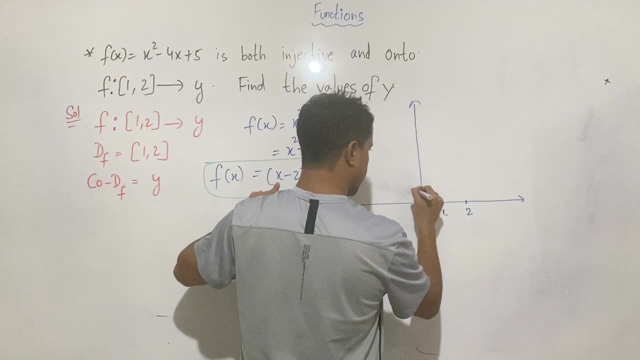 going to be 0 and this thing is going to be 0 when your x is going to be 2.. so when your x is going to be 2, then value of y is going to be 1.. so this is 1, this is 2.. so at 2, value is going to. 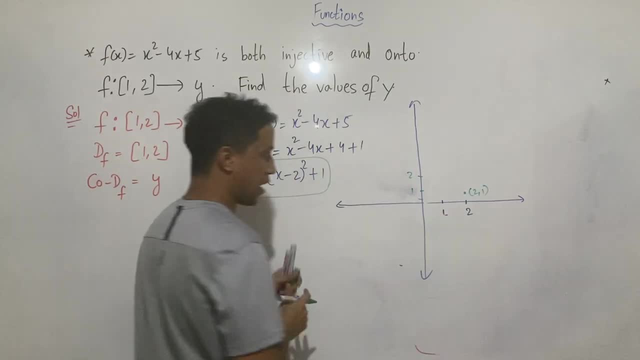 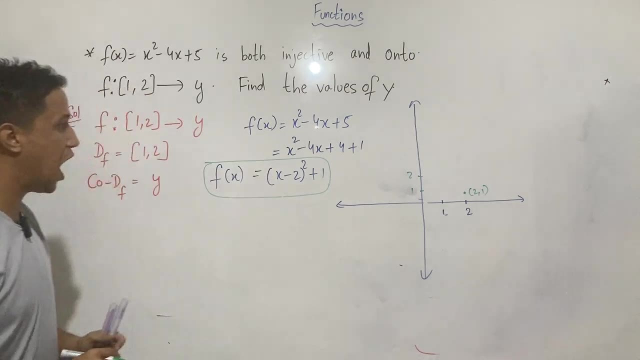 be 1.. so here, 2, 1, right. so because this is defined from 1 to 2 closed interval. so what's- let's see what's how it's going to behave at one. if you put one here, then the value of this function is going to be 1.. 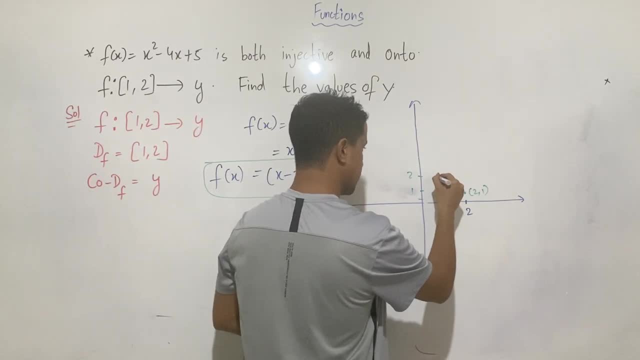 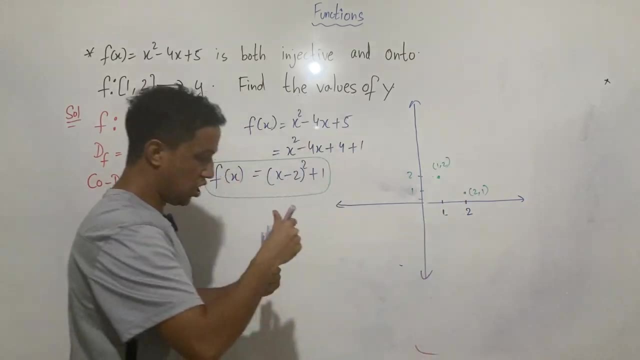 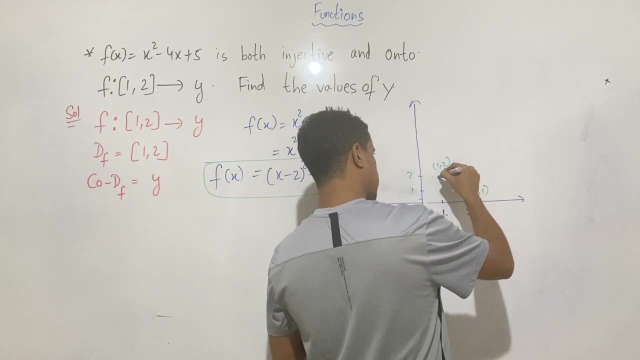 going to be 2. 2 so means this. this means here, 1 at 1 value is going to be 2.. so see here, this graph will be like this. it's going to be like this. okay, now i have to only deal in this interval. 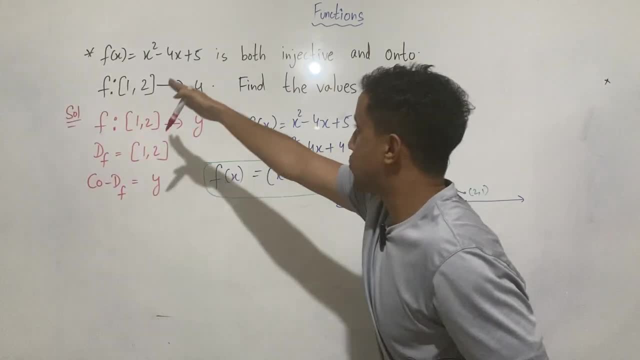 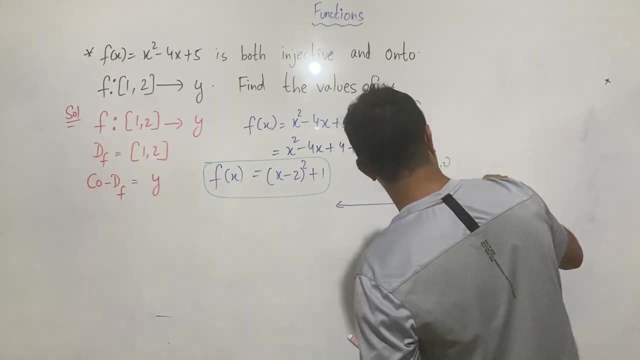 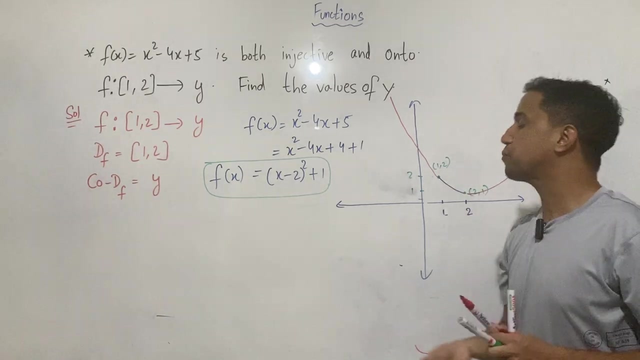 what i am trying to say here is that if it is from real number to real number, if this is from real number to real number, then this graph could have been like this, like this, like this parabola. but i'm not interested in that, because it says that 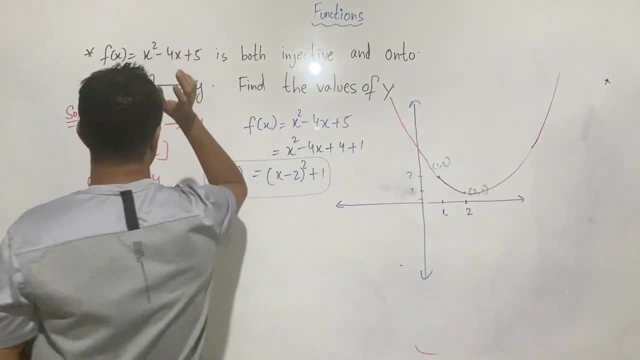 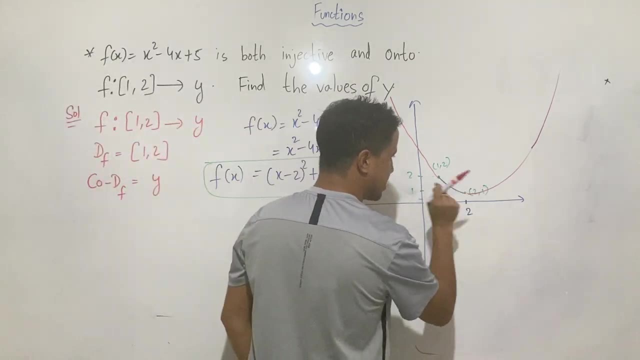 only in this interval. this graph, sorry. this function serves as both injective and onto injective here, in this interval it is. injective means this is 1, 1. so if you draw any horizontal line here then it will be 1, because this is zero. so you get 1, 1.. so this is 1, 1.. so in this case, 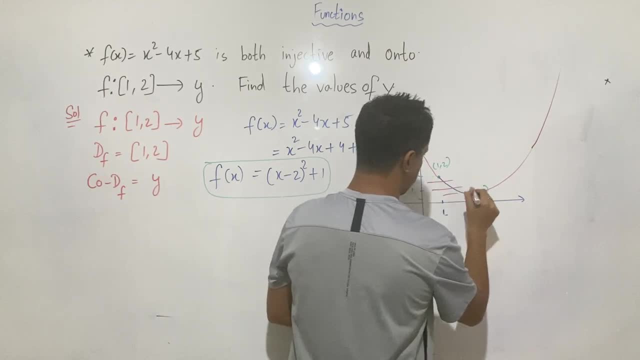 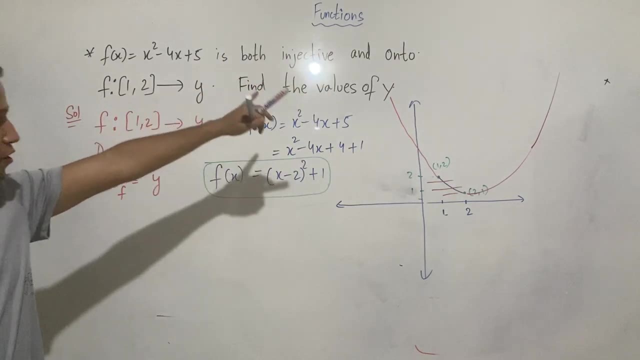 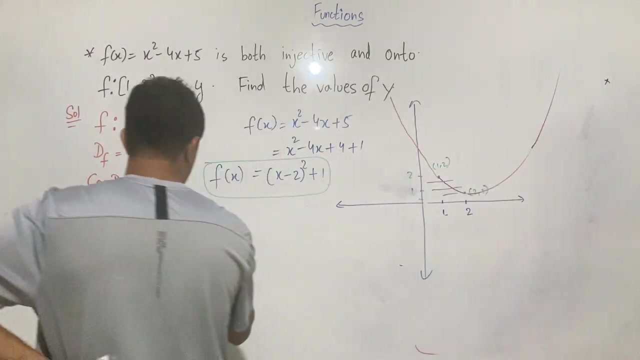 then it's just going to pass through once. So this is injective in this domain and onto. Okay, so this function is also onto here. Okay. so if it is onto here, then what Then? if it is onto, then now see here: if it is onto. 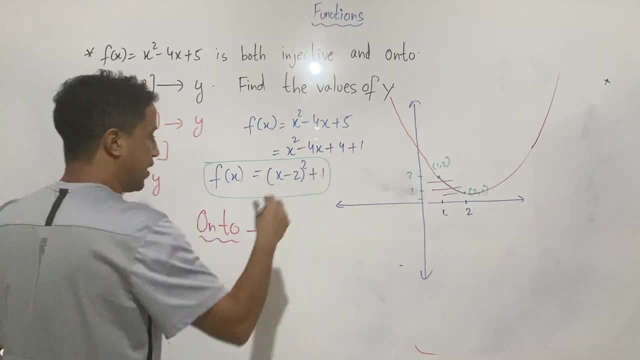 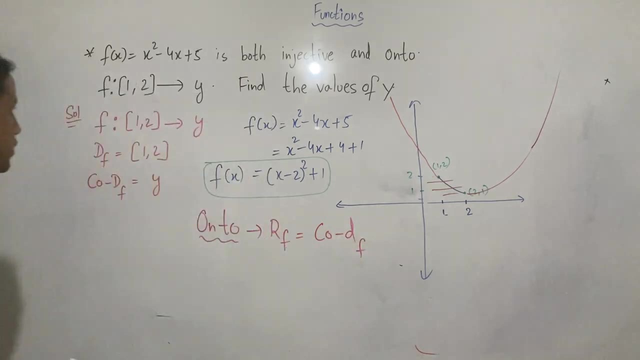 Okay, let's see. if it is onto, then what? Then? your range is going to be your codomain- Am I right Codomain? And what's going to be the range? Now you check in this interval. Okay, this interval. 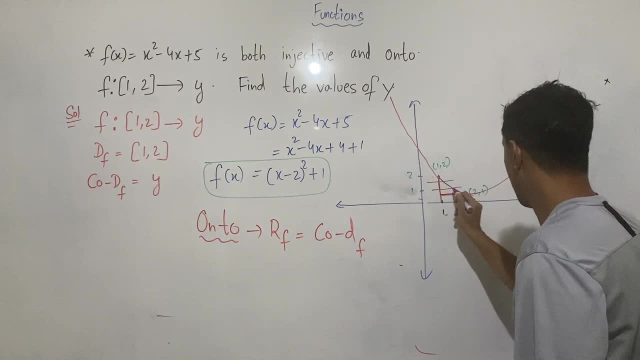 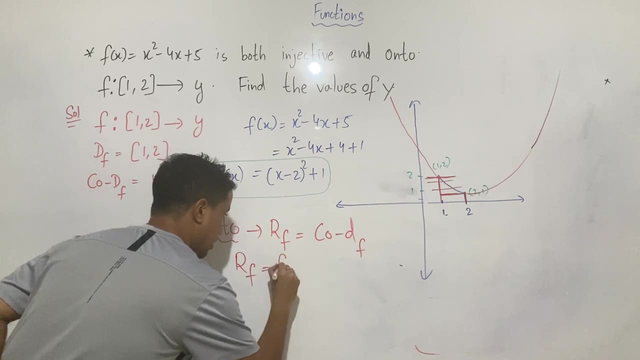 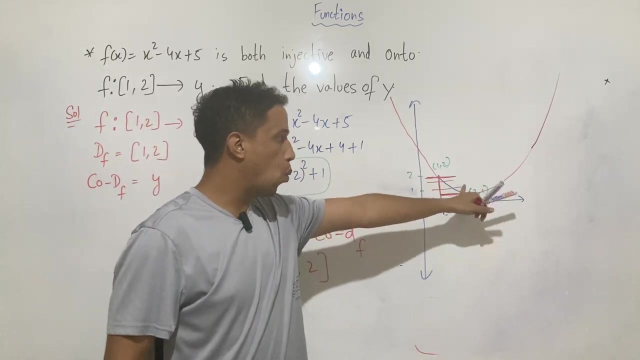 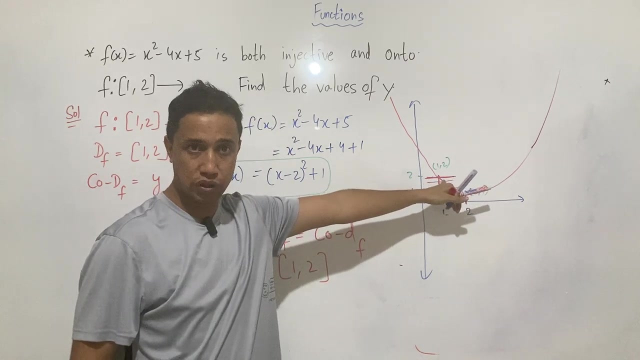 See, here this is going to be between one and two, Right? So your range is going to be one to two. closed Interval, because that's the value of, that's the value of Y at two, and here the value of Y at one, X equal to one. 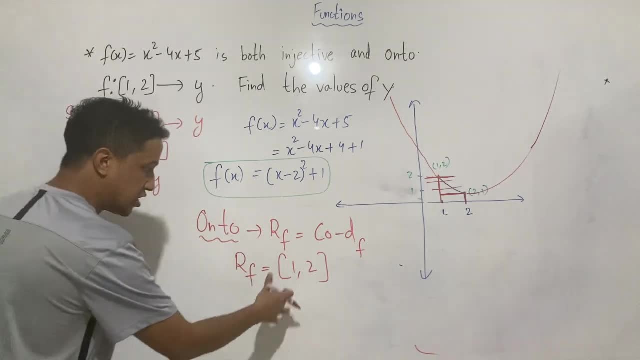 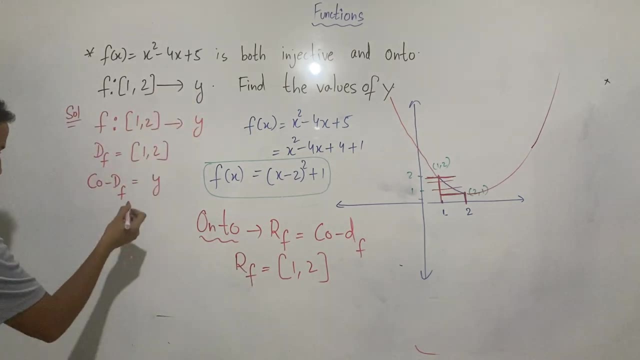 So this is going to be the range. So we know that codomain is similar to range when your function is onto. So what does it mean? It means your codomain is Y. So from here, here we can say: therefore, therefore, you're. 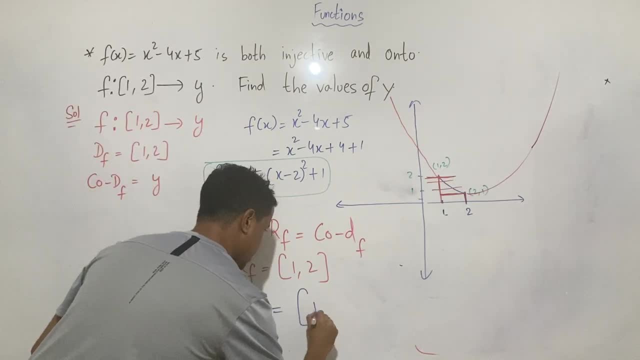 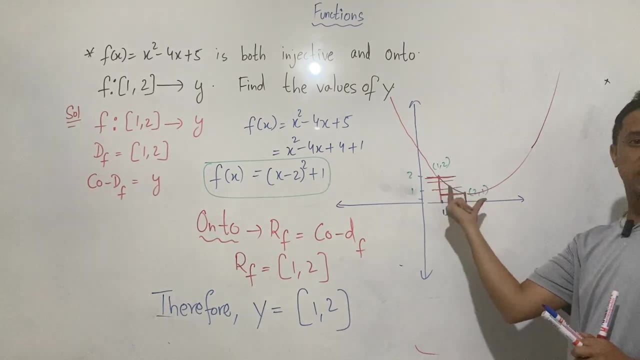 Y, it's going to be in this interval. I hope it made sense. This is a nice question. Okay, because you just have to deal in this interval. Okay, so that's how you have to do it. Okay, you can just have a look. 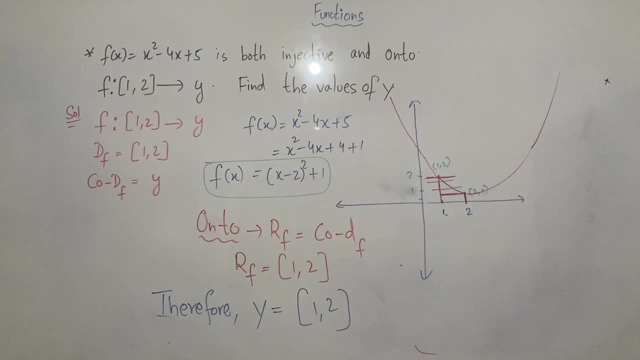 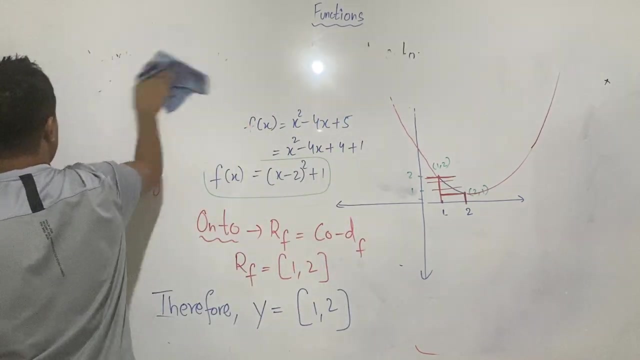 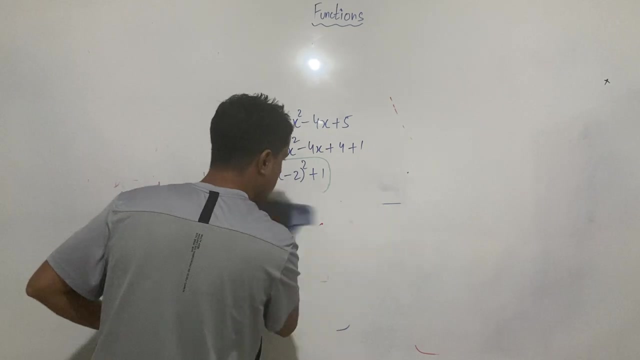 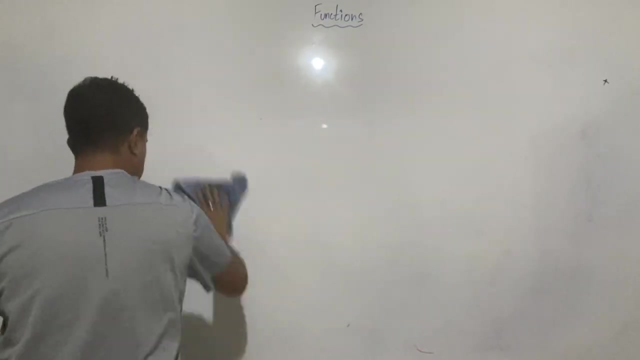 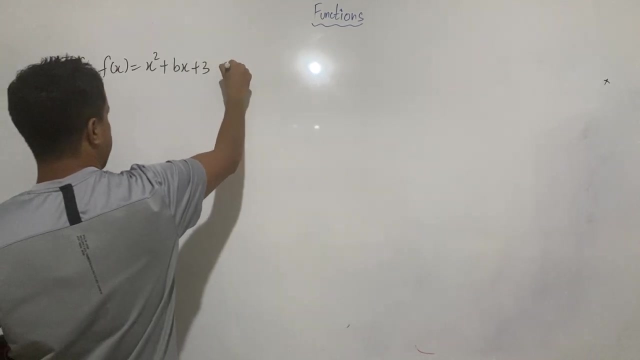 And if there is any doubt, just let me know. Okay, Now one more question. Okay, so write down the next question. The next question is: it is If, If your function of X equal to X, care plus B, X plus three is not. 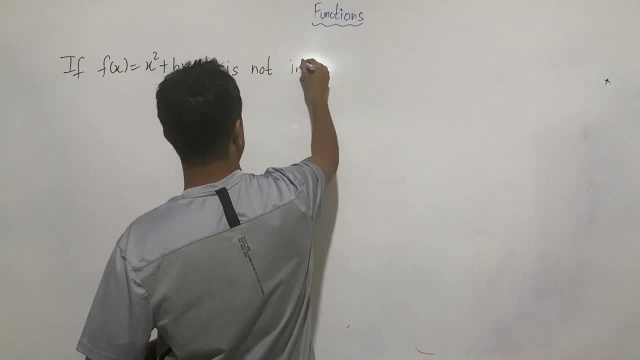 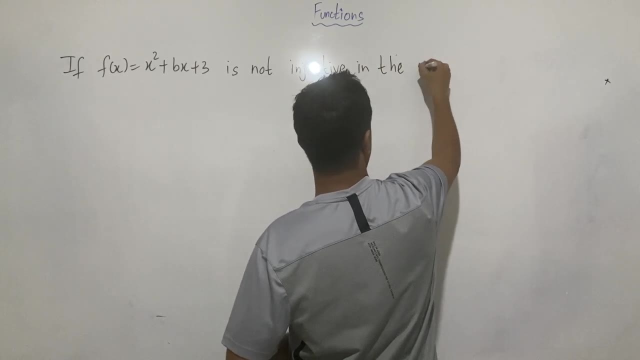 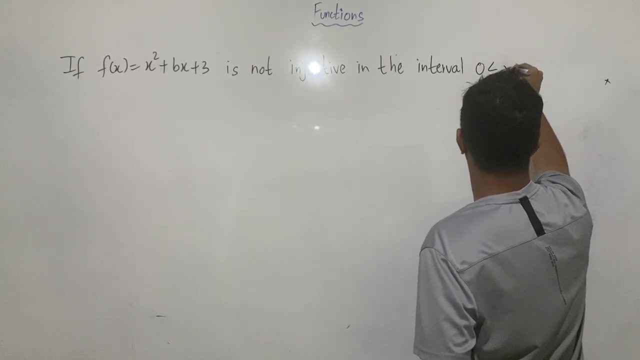 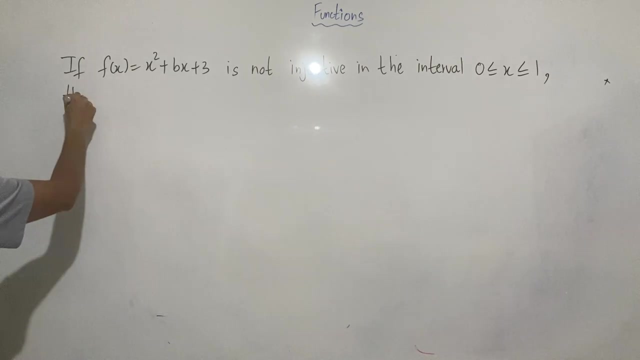 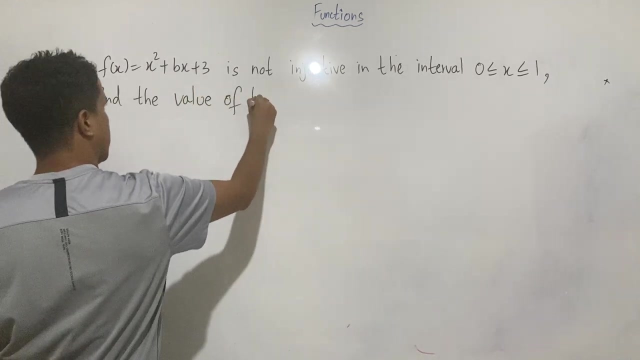 If it is not injective, Injective In the interval, in the Interval, What interval? zero to one, Okay, Zero Two, One, One, Then Then find, Then Find the, The value of B, Okay, now, this is also a nice question. 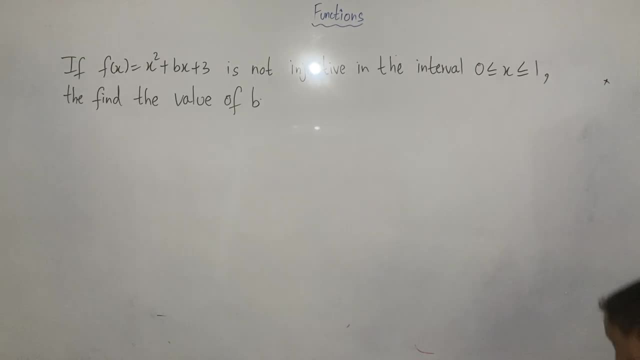 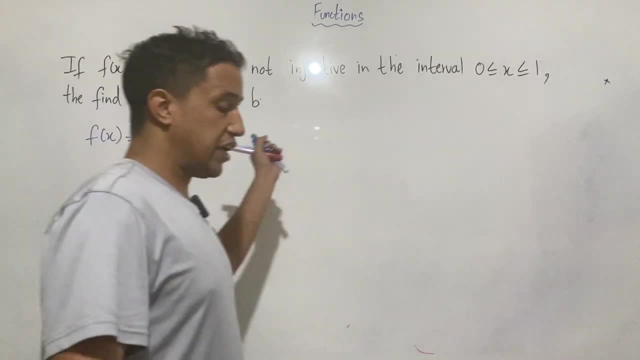 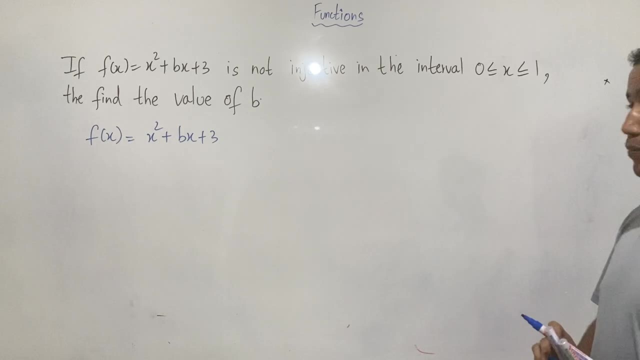 This is. This is. This is three. okay, so if you look at the type of function, this is quadratic function, right? so i am sure the graph is parabola, right. so here it's going to be para bola. but here my main concern is interval 0 to. 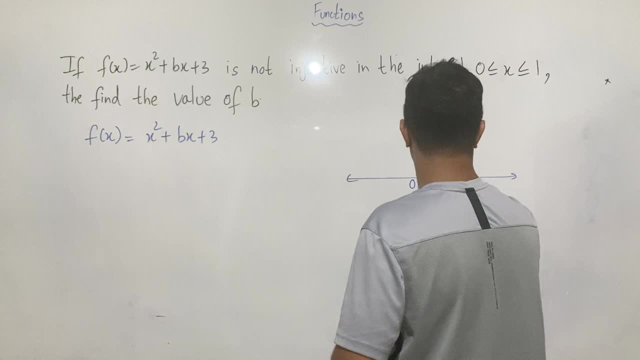 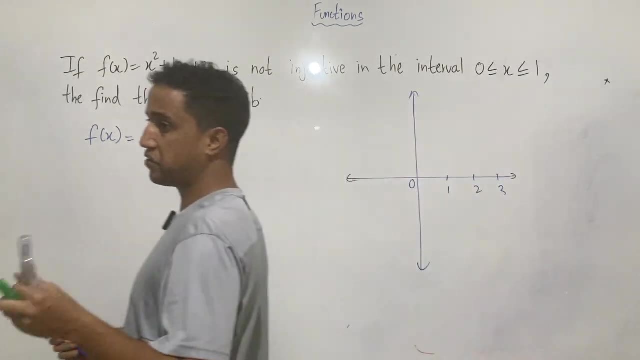 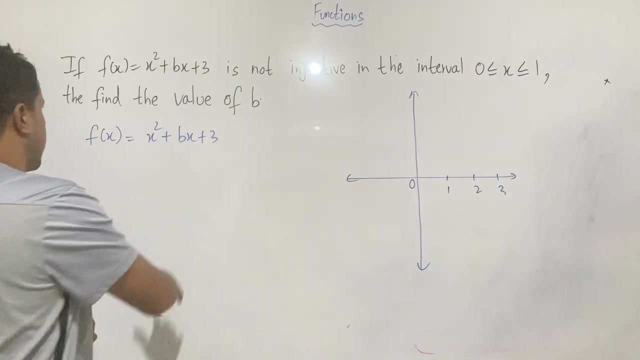 1. right, so let's say this is 0, this is 1, okay, here it is 2. but these points are not of my concern. i'm more interested in behavior of this function from 0 to 1. okay. now here the given function is this: 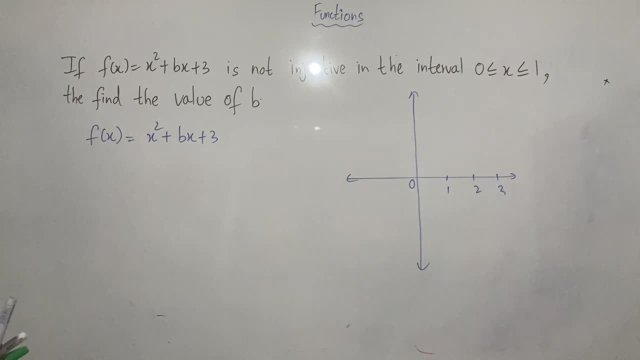 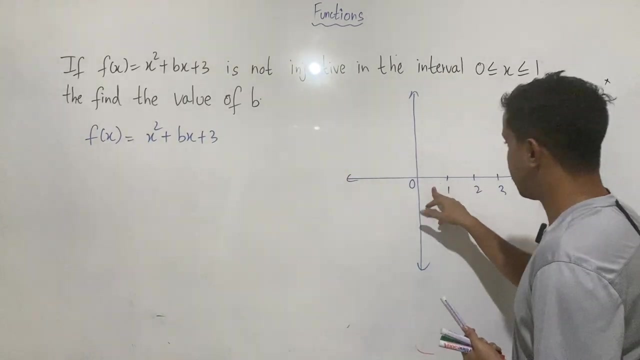 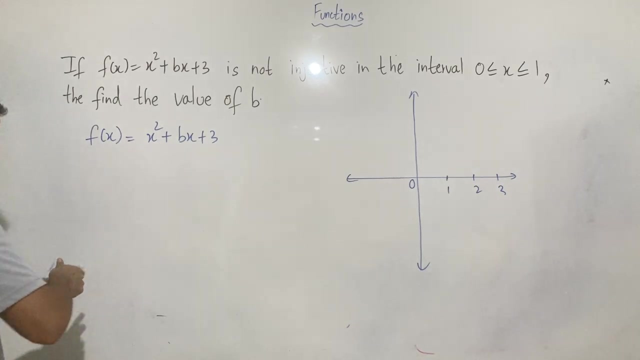 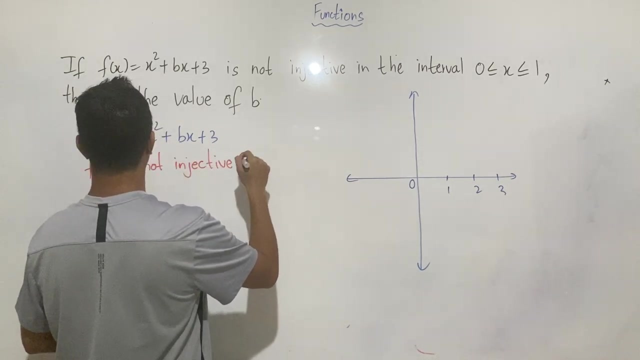 okay, we have to find the values of b. okay, now, if this function is not injective in this interval, okay, not injective means that this function now see here, fx is, fx is not injective, right, fx is not injective, injective m. fx is not injective for. 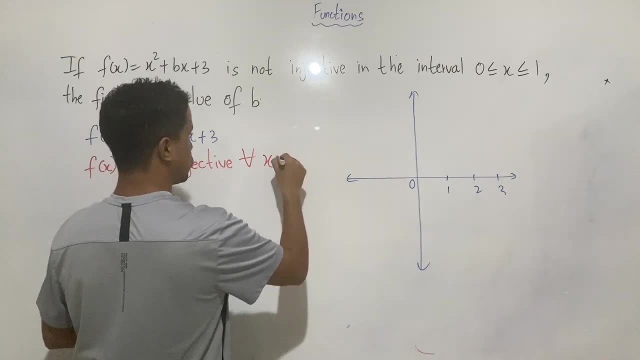 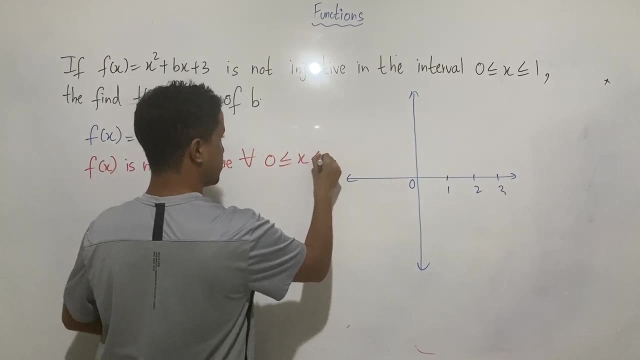 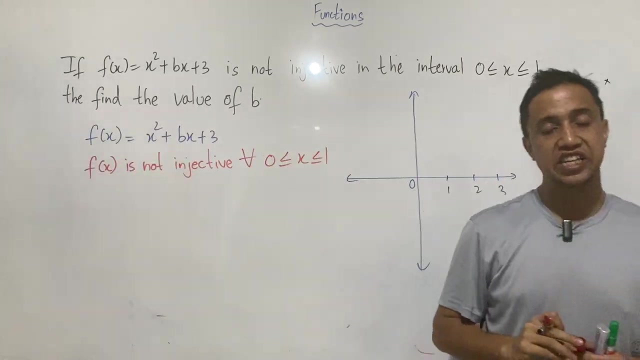 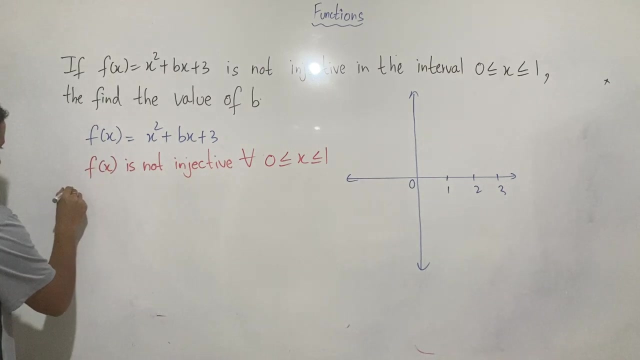 all x belongs to uh to. for all x belongs to x belongs from 0 to 1 right. what does it mean if it is not injective? if it is not injective means one one, then it means it is many one right. so which means therefore? therefore, fx is. 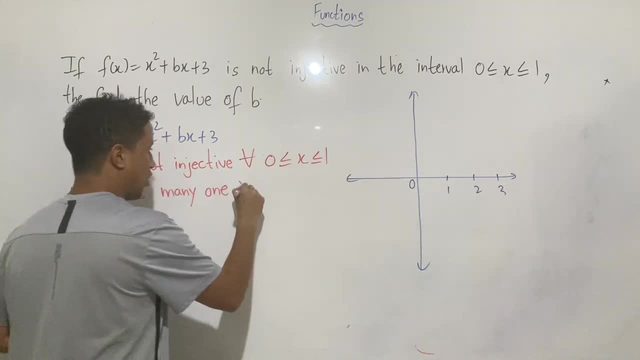 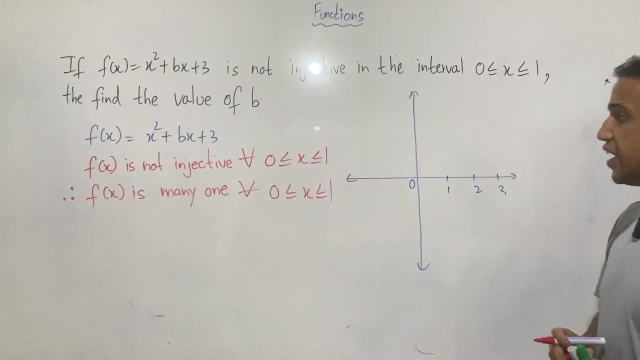 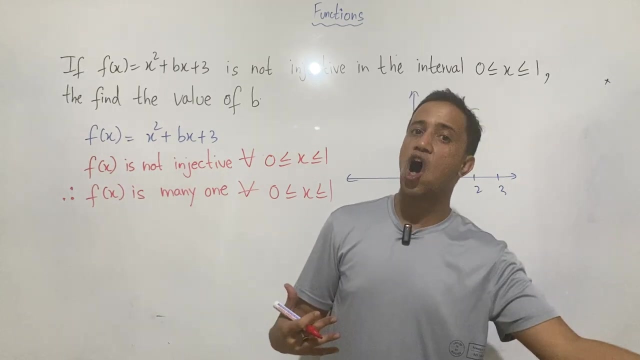 many one, manyb, many, 1 for all. x belongs in this interval. okay, So if it, I have told you: if function is not injective, then it means it is many 1.. If function is not onto, it means it is into right. So 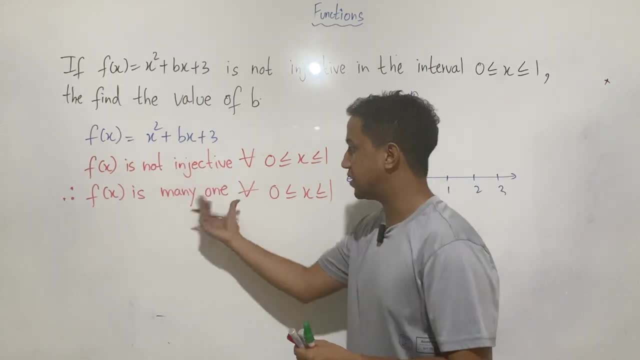 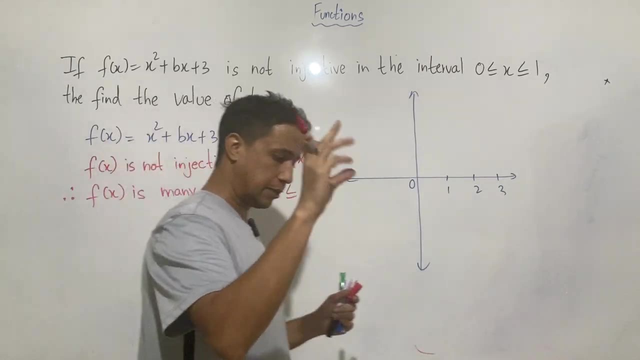 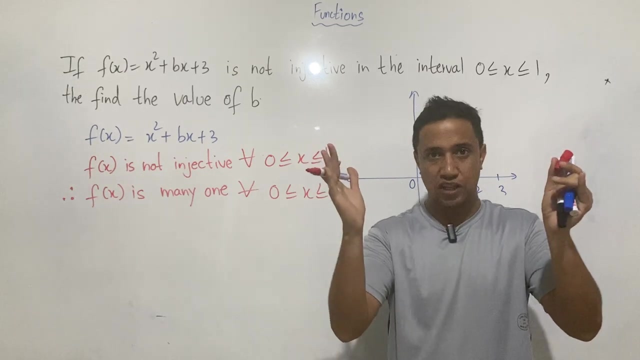 same here. if it is not, injective means, if it is not 1, 1, it means it is many 1, right Now, many 1,. what does it mean? Okay, many 1 means that that for two values of, for two values in. 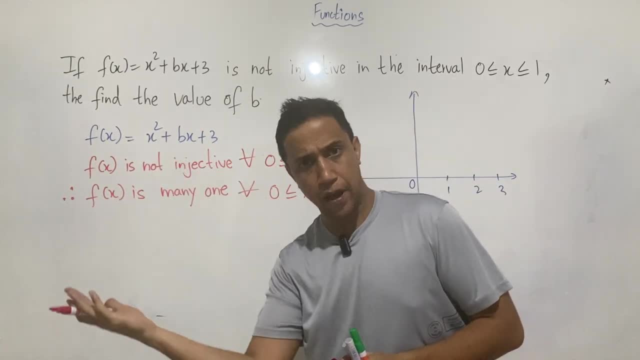 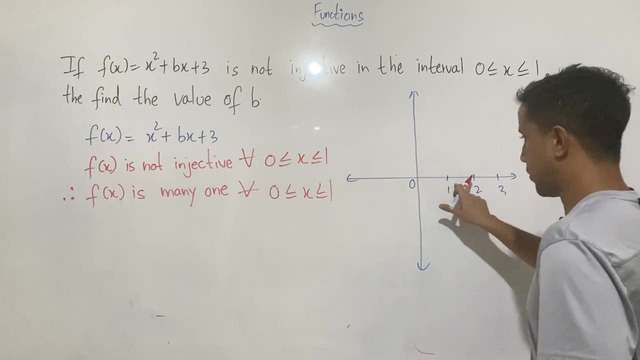 domain, you can get one value in the range, right? That's what it says. Now, see here. So if it is here, right, if it is here, it means it has to be. it has to be many. 1 here. 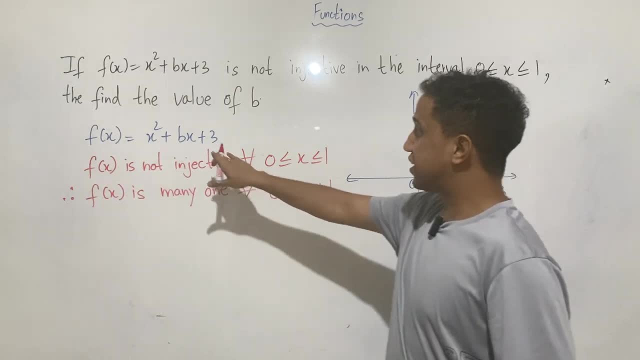 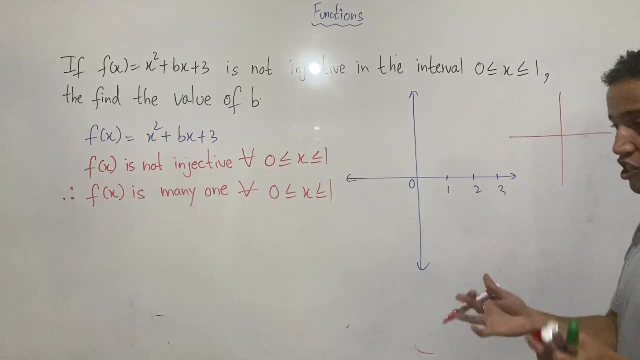 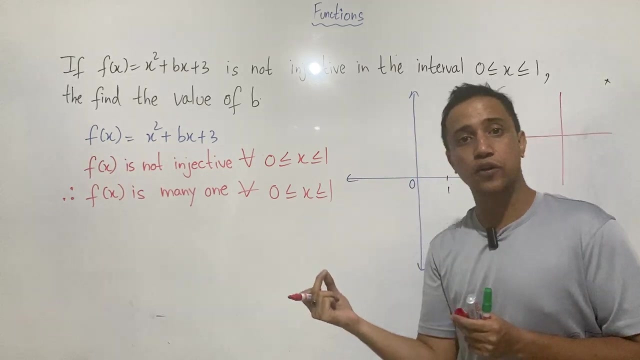 in this interval. Okay now here the thing is that if you look at any quadratic graph, okay now, where the possibility? what's the possibility of, of, of, of, of getting function as many? 1 when the given. 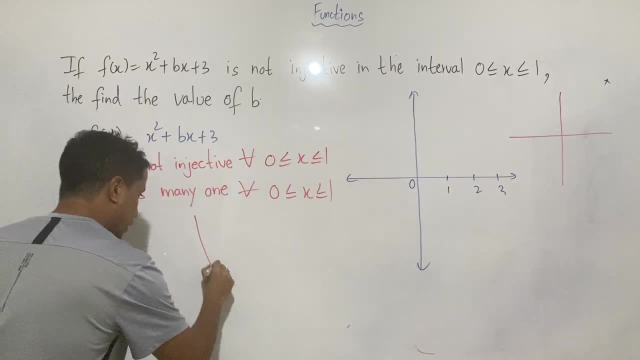 function is quadratic. Now see here, it's parabola, right Parabola. So the only chances is that when you get this part, where if you draw, for example, see here, if I draw any horizontal line, horizontal line here, so the chances are that in this interval I can see. 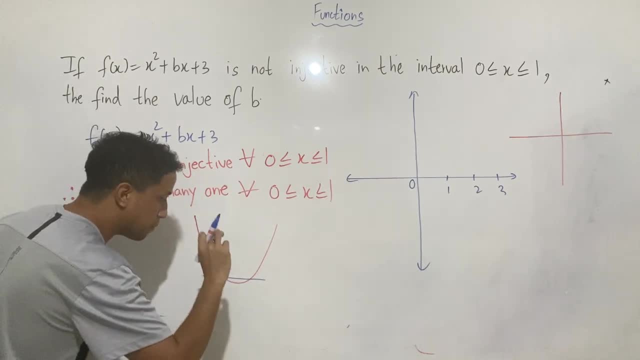 this many 1 nature, right. But if you tell me, for example, here this is x equal to 1,, this is x equal to 5, okay, So in this interval from 1 to 5, you can see, I can draw any horizontal line. 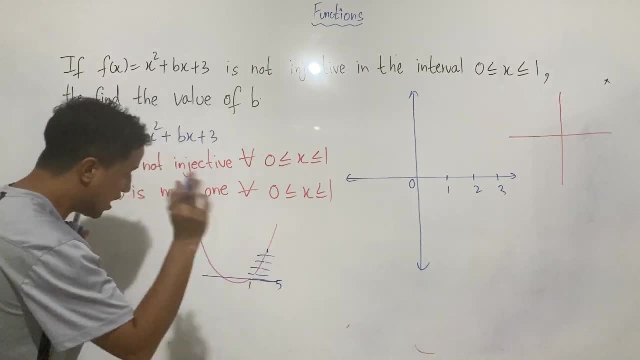 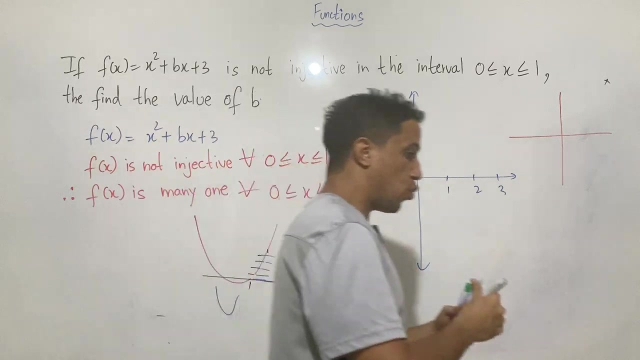 this function is still going to be 1,, 1, right. But the interval, this is the interval where you will get the lowest point right, Where you will get the lowest point. Now, we know that. now, see, see here. we know that. we know that the the lowest. 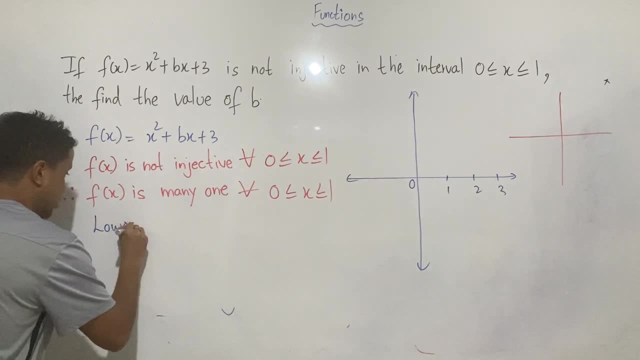 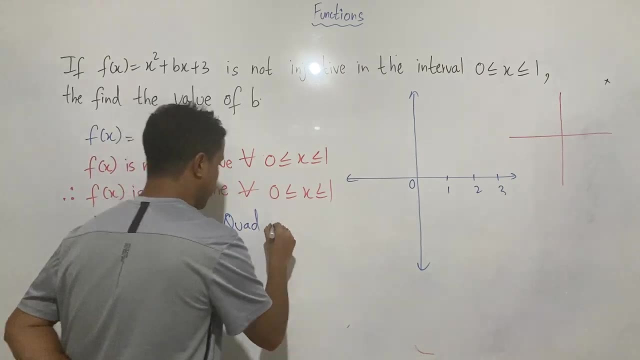 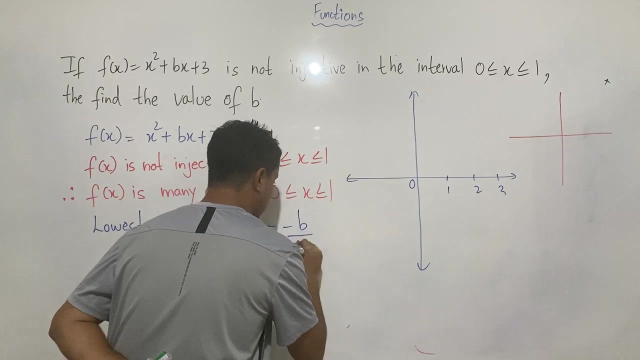 point right, The lowest point. the lowest point point in quadratic. okay, In quadratic, what's the formula for that? The formula is x. it is x equal to minus b over 2a. okay, So if you. 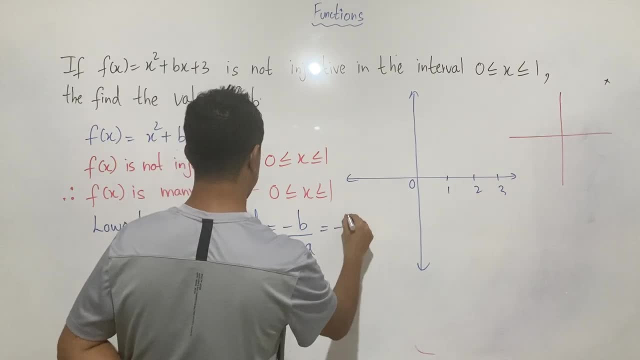 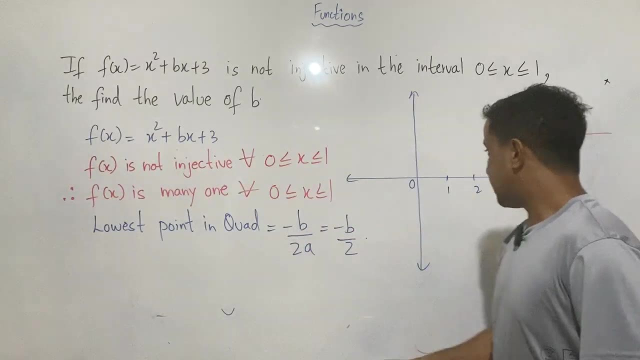 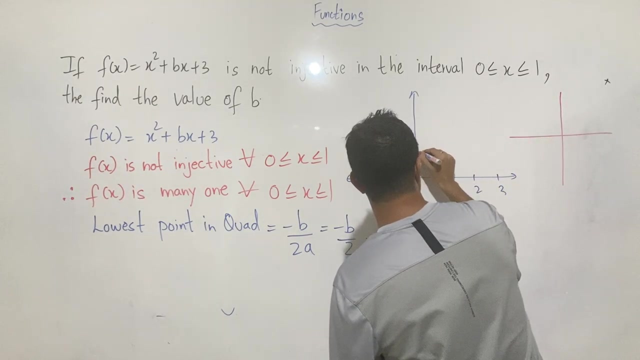 do it here. it's going to be minus b divided by 2 by 1, minus b by 2, okay, So the lowest point it's going to it has to be between 0 and 1.. Why? Because, see here, if it is going to be between 0, 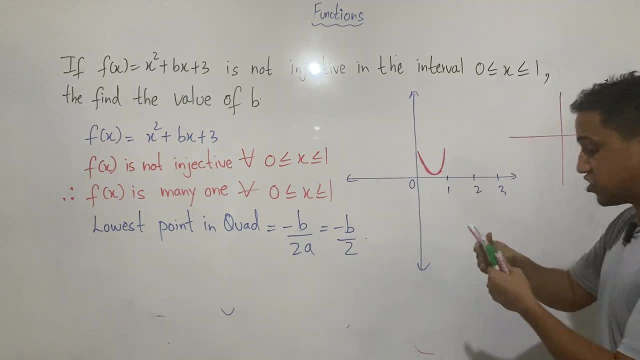 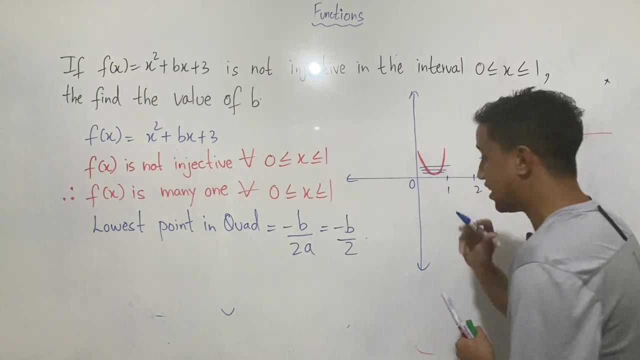 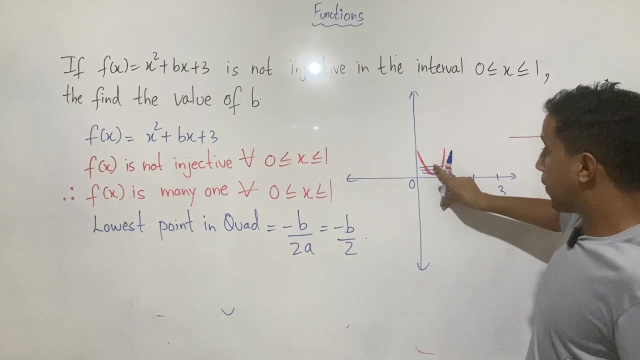 and 1, the lowest point. then this is the point where the possibility of this function as many 1 is more right, Because, see, here this is going to be many 1, only in this region. Why? Because if from this region to here, this is going to be 1, 1.. And again the same thing. this is my parabola. 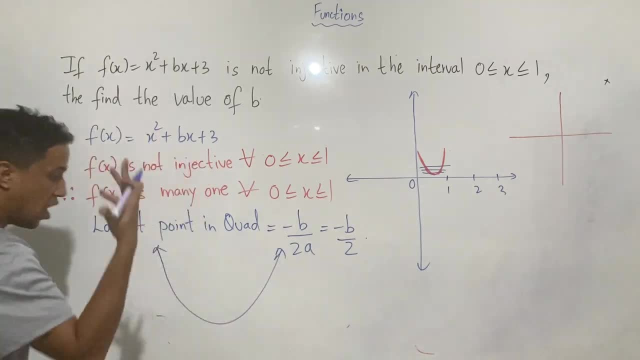 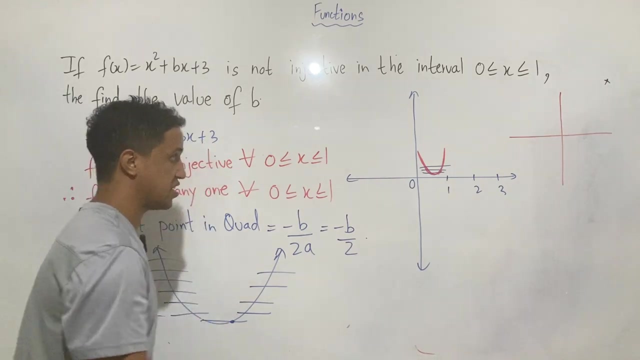 okay, The possibility of many 1 is more when I am here- See here, because the horizontal is cutting this curve more than once. okay, But after here it's cutting just once. The chances are negligible Here the chances are almost none. So the only chances is where I will get the lowest point of 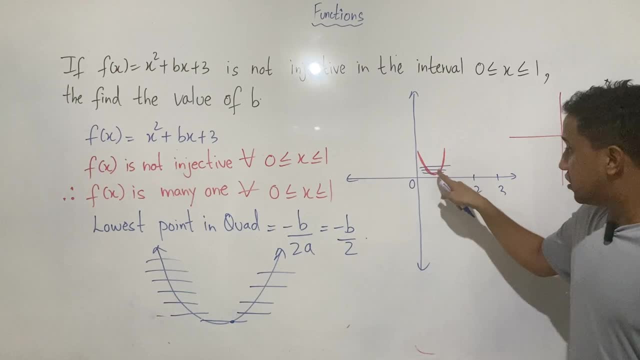 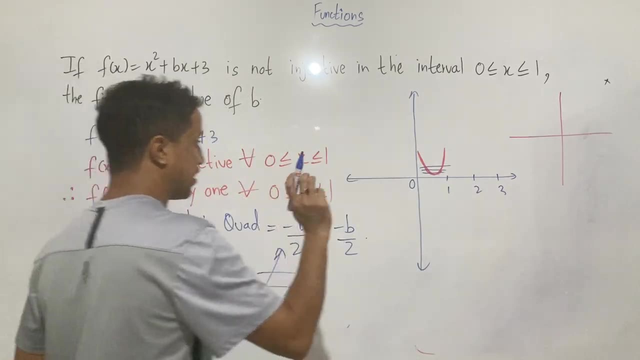 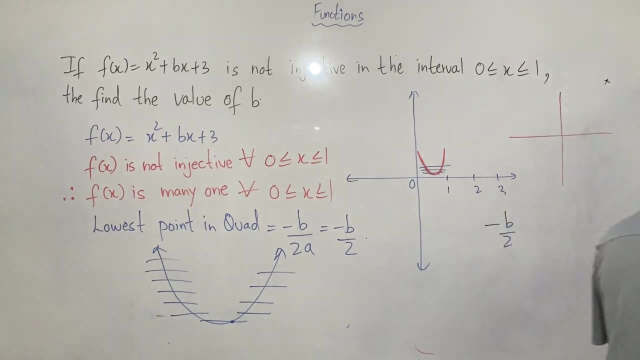 this upward parabola, which means that this lowest point it has to be somewhere between 0 and 1, right, So I can say that this point minus b by 2, okay, It has to be between where Between 0,. 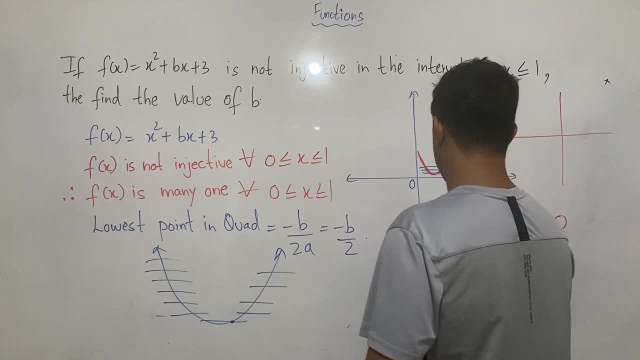 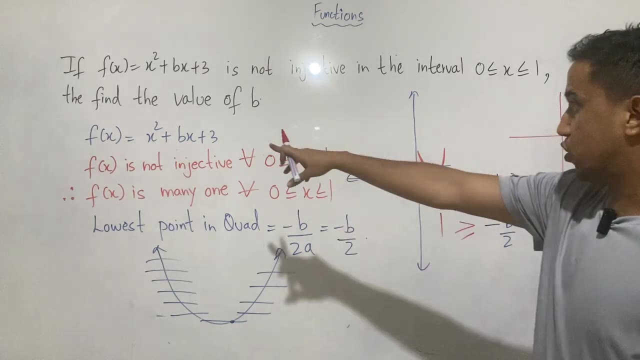 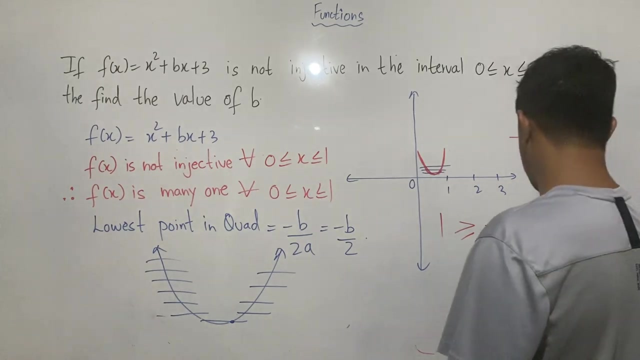 0 and 1, right. So if that happens, then how do I get the lowest point? Well, I can say that I can find the value of b. So if I multiply it with minus 2, then here I will get b, here what? 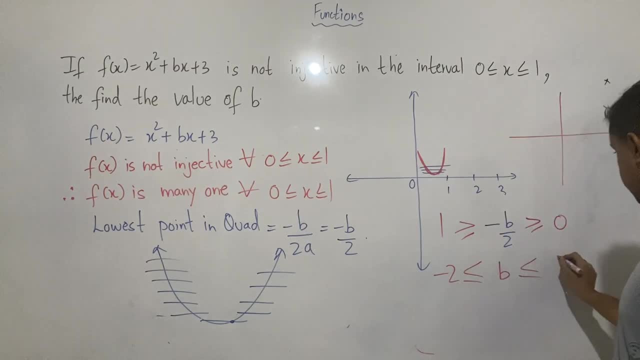 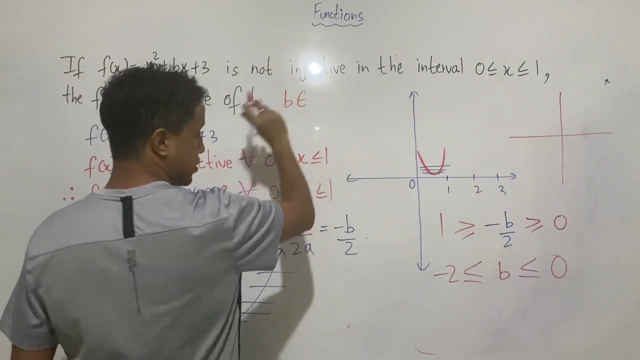 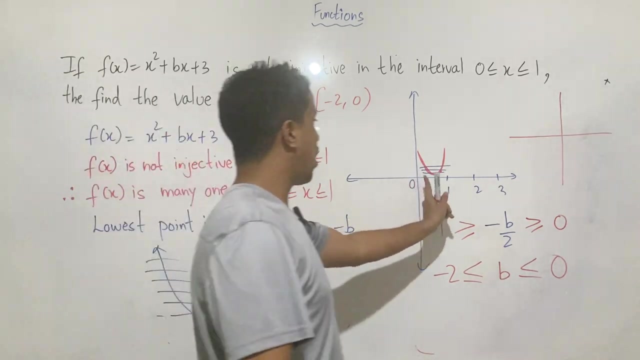 Minus 2, right. Minus 2 to 0, right. So your b, the value of b, it is going to be in the interval minus 2 to 0.. Okay, So here, because we are interested in this, 0, 1, it is not injective here means that it is. 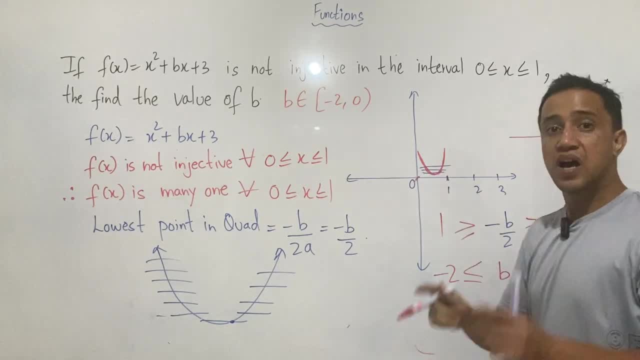 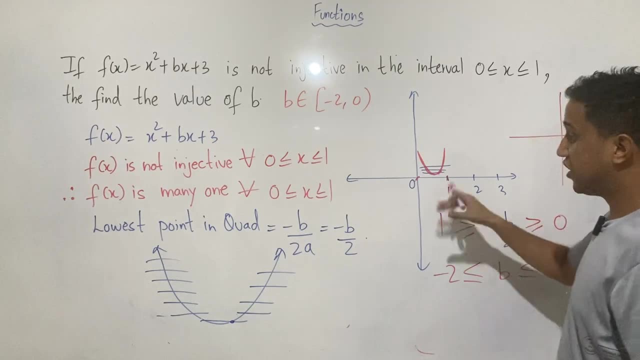 many 1 here The chances, how it can be many 1, the lowest point has to be formed between 0 and 1, anywhere between 0 and 1.. So we know the formula to find the lowest point which, if you don't know, 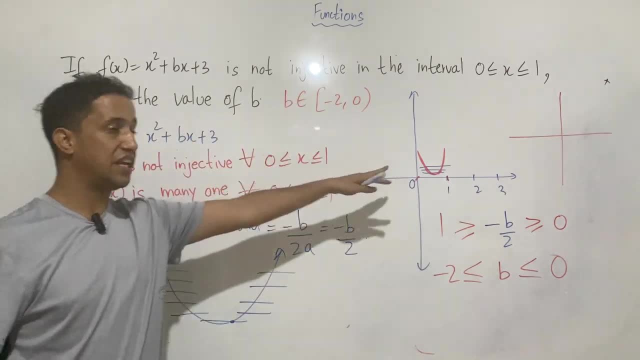 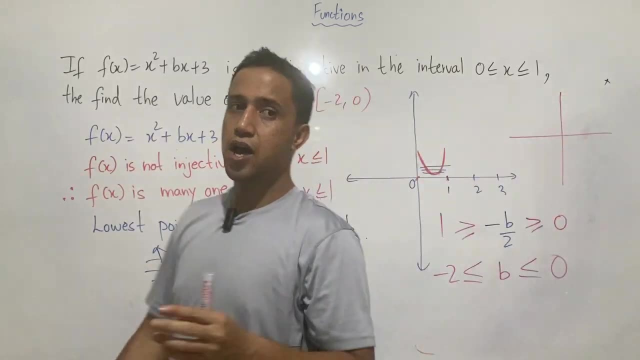 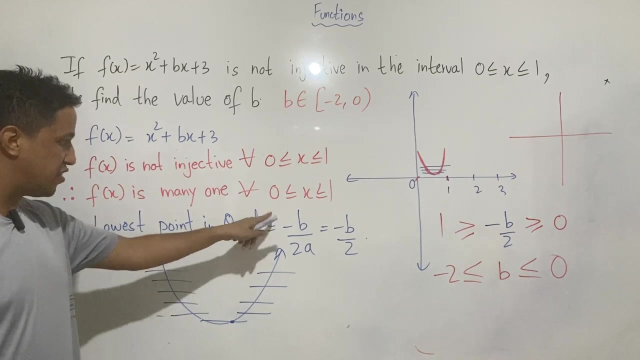 then yes, you have to know that right Later on in the application of derivatives, we are going to to talk a lot more on that point of minima, point of maxima. But just remember the lowest point, it is obtained by this formula: x equal to minus b over 2a. So when we substituted the things 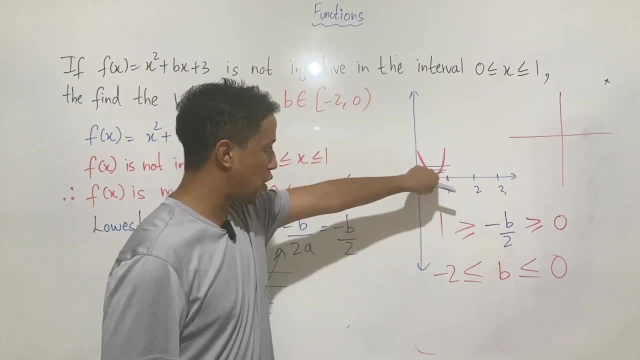 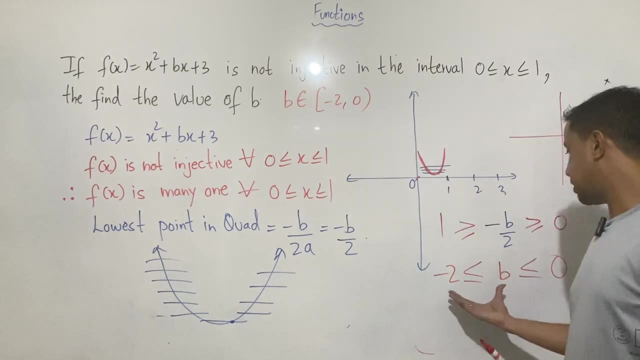 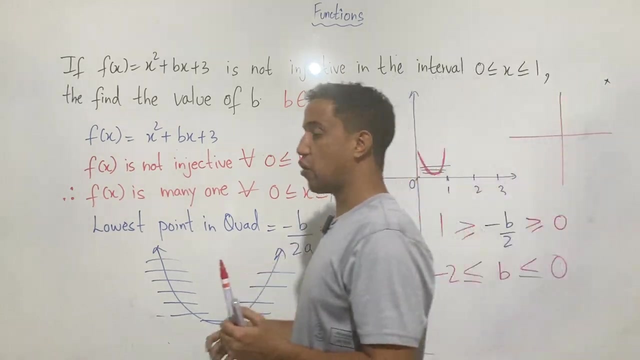 and then when, here I said that lowest point it has to be between 1 and 0, right, 0 and 1. So when we, when we simplified it further, then we got the value of b in this interval. Okay, So that's how you have to approach the problem. 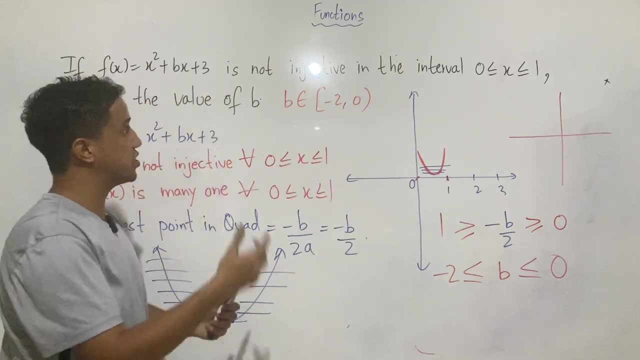 So I hope you have clarity on this onto and into functions. Okay, So we'll see you next time. Thank you very much, Keep safe, Have a great time. Bye-bye.